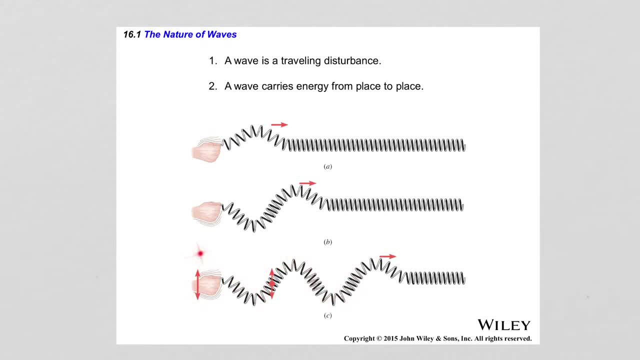 multiple disturbances are created each time the hand goes up and down, and those disturbances are going to travel away from the hand. So waves are traveling disturbances. Furthermore, the motion of the hand up and down imparts energy into the wave. The motion itself requires energy. 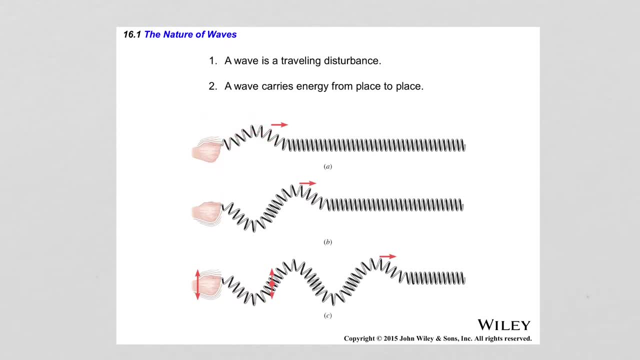 so this energy is transferred to the wave, And so, as the wave moves away from the source of disturbance, this energy is carried down the medium, And so energy can be transferred by waves from place to place. A very simple example that will illustrate that point would be the energy that we get from the sun. 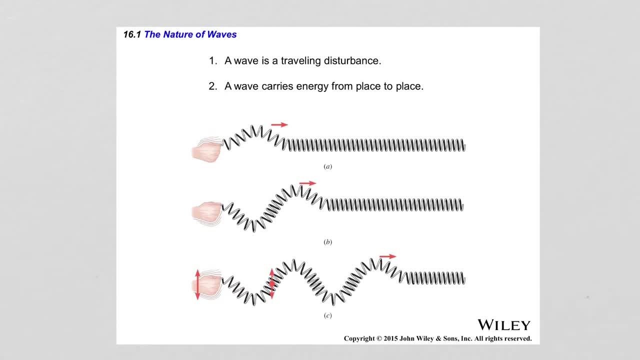 The sun emits electromagnetic energy, Which consists of microwaves, x-rays, visible light and a large variety of other waves within the electromagnetic spectrum. So this energy carried by these waves reaches us and we feel that as warmth. So you know that when you get under the sun you feel warmth. 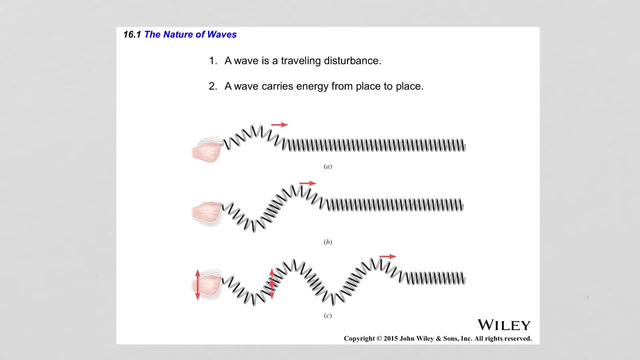 You get in the shade, You don't feel as warm. So that's an example of energy being transferred by waves. We have two main types of waves, based on how the particles of the medium oscillate when a wave is created in that medium. 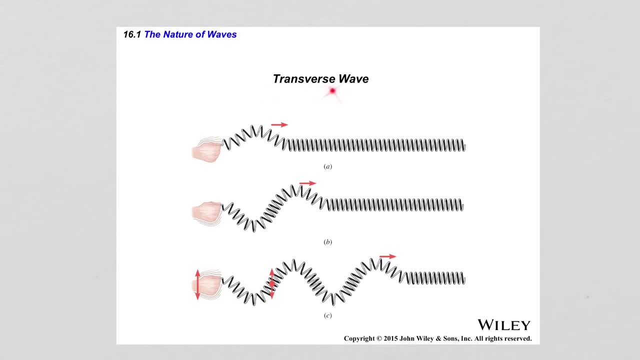 The first type of wave is the transverse wave In the slinky. here a disturbance is created by shaking the free end up and down, And so as the disturbances are created in the slinky, we can see how the slinky itself is not moving away from the source of the waves. 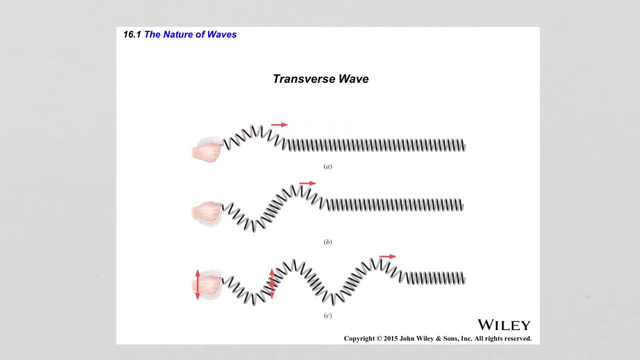 The hand does not lose the slinky. The slinky doesn't pull from the hand. The slinky doesn't pull from the hand. Instead, what happens is the particles of the slinky oscillate up and down as the waves pass through those particles. 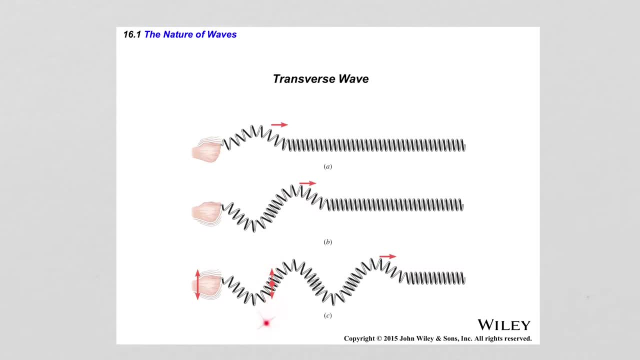 And so the direction of oscillation of the particles of the medium, in this case the slinky, is perpendicular to the direction of propagation of the waves in the slinky, And that's why these types of waves are called transverse waves. 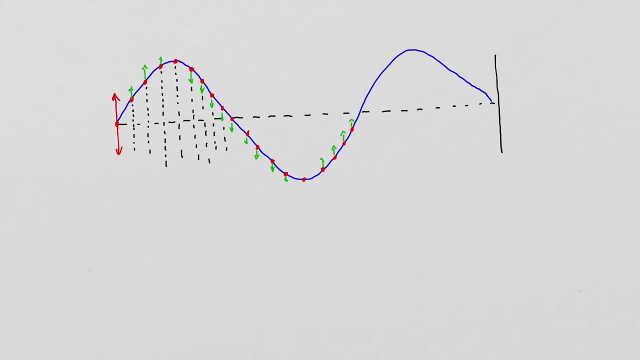 Let's illustrate this concept With another medium, and that is a rope. So when the rope is stretched and there are no disturbances created in the rope, the rope is obviously horizontal, like so If the far end is attached and the free end is where disturbances are created, 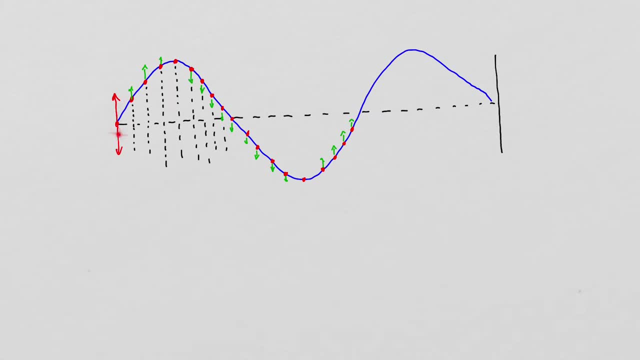 once the free end is moved up and down, waves are created in the rope, And so here we have three waves that are created in the rope, and these waves propagate away from the source of disturbance. So here I have indicated several points. 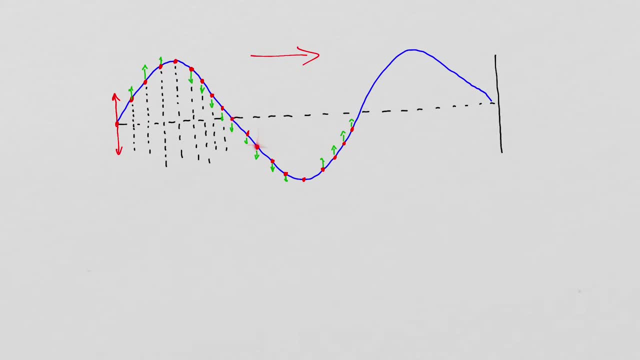 or particles, rather, inside the rope, And so, as you can see, as the wave passes through the particles, they move in different directions depending on where the wave is along the rope with respect to these particles. So, for example, this first particle is moving up. 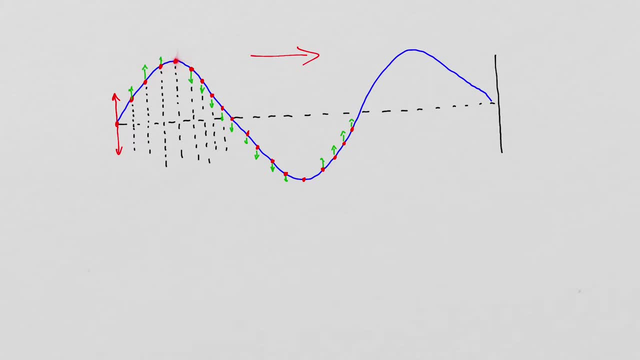 the next one, also moving up. the third one is moving up. the particle at the very crest of the wave here, however, is stationary, And then, after that, the particles behind they start to move down and down, and down and down. 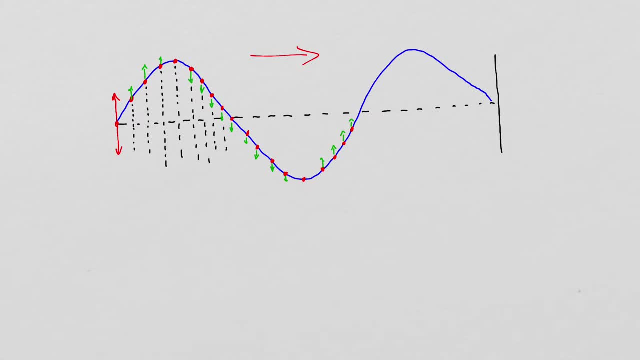 until we reach the very bottom of the trough. here this particle is stationary. After that the particles are starting to move up, and so on and so forth. So if you trace the motion of these particles, you see that they are moving. 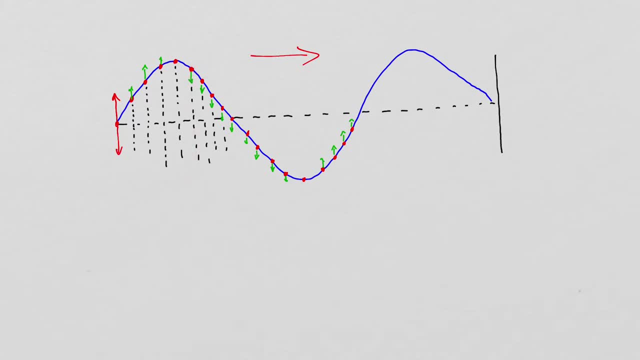 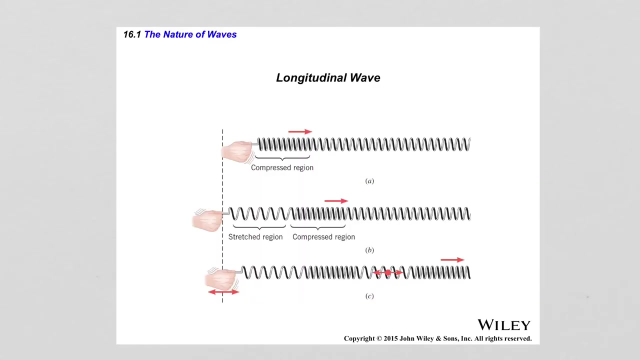 in a vertical direction, here, up and down, while the waves are moving in a horizontal direction, away from the source, And so, again, that is why these waves are called transverse waves. The other type of waves are the longitudinal waves, Again. 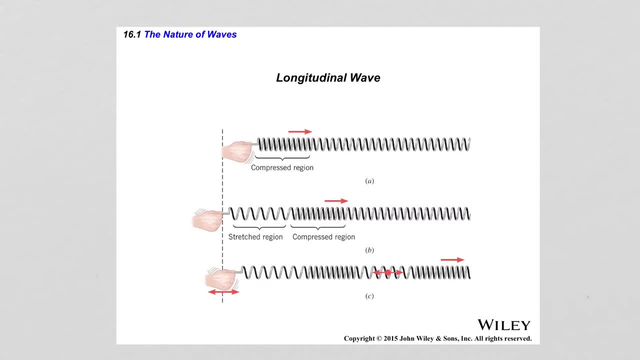 the example I will use about the longitudinal wave is a disturbance created in a slinky. The difference from the previous example now is that the hand here is pushing and pulling on the slinky. So if the hand pushes on the slinky, a region 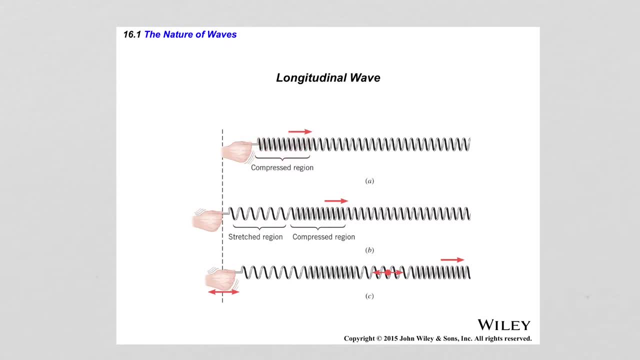 of compression will be created in the slinky in the immediate vicinity of the hand. After that, the hand pulls on the slinky and a region of stretched slinky will be created in the immediate vicinity of the hand. And so now we have two regions. 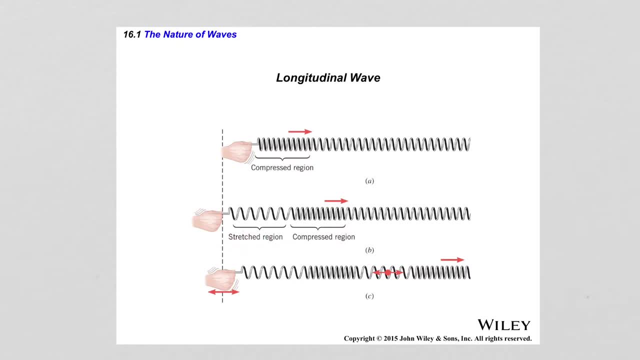 We have a region of compression and a stretched region. If the hand continues to move back and forth like so, multiple compression regions will be created or multiple stretched regions will be created, And so this now is a series of waves that propagate away from the hand. 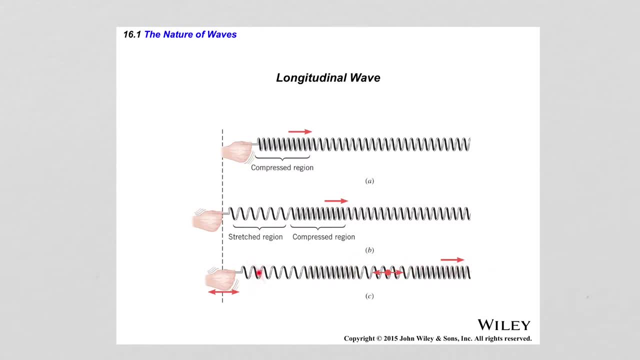 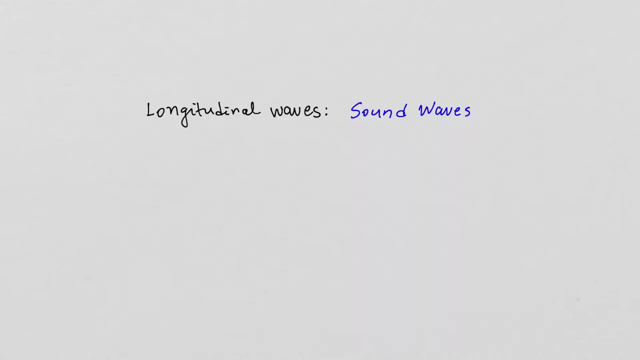 down the slinky, but the particles of the slinky also oscillate in the same direction, or parallel, rather, to the direction of propagation of the wave, And so therefore, the name is longitudinal waves. An example of a longitudinal wave. 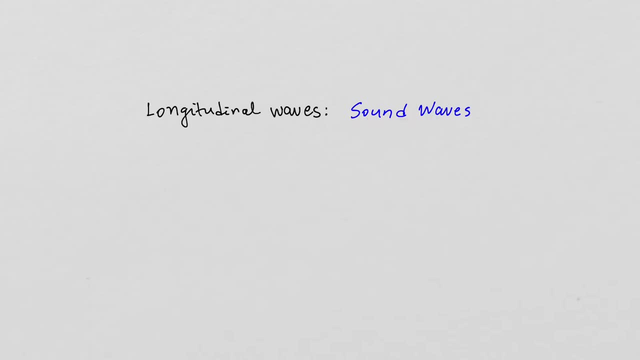 would be sound waves. Of course, I talked about waves created in the slinky, but that is a very specific example just to illustrate the point. In real life, the most common example would be sound waves. For transverse waves we have a lot more variety. 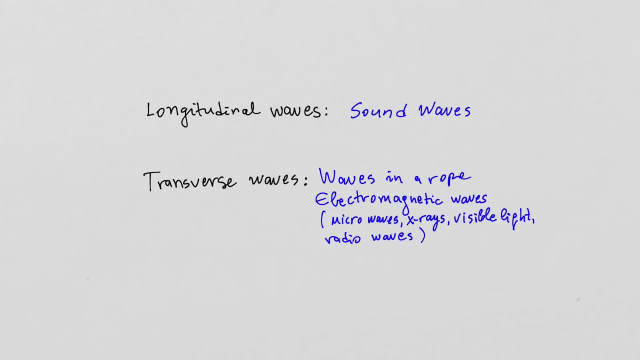 of waves. The most prominent ones are waves in a rope, or also the waves created on the strings of musical instruments, and also electromagnetic waves. The electromagnetic spectrum is a very wide spectrum of various waves. The ones that are most commonly known are microwaves. 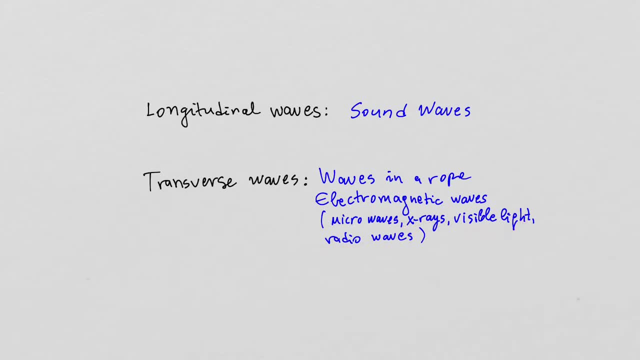 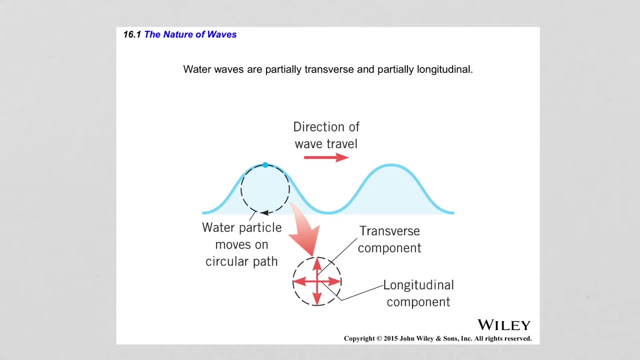 x-rays, visible light and radio waves. There is one interesting example of a combination of longitudinal and transverse waves, and that combination is seen in water waves. So here is a set of two water waves which are propagating to the right. 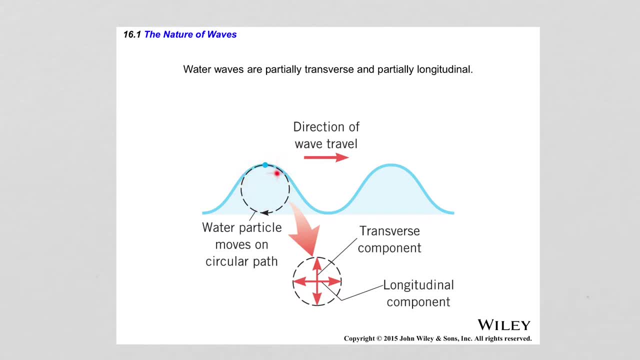 and inside each of the waves there is a circular motion generated by the combination of a longitudinal component and a transverse component. And so if you have been in the ocean when there are waves, you know that the waves travel towards the shore and also you feel that. 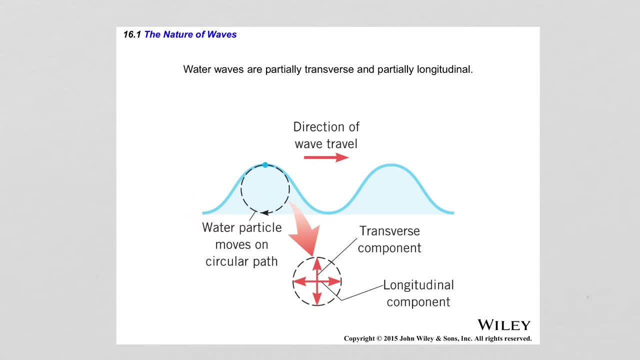 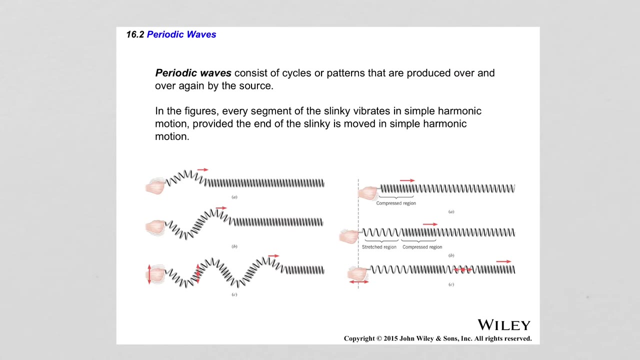 at the bottom, you feel like a pull towards the depth of the ocean, And this is because of the combination of transverse and longitudinal components of the waves. What happens if multiple disturbances are created in medium and those disturbances are exactly identical to each other and are created? 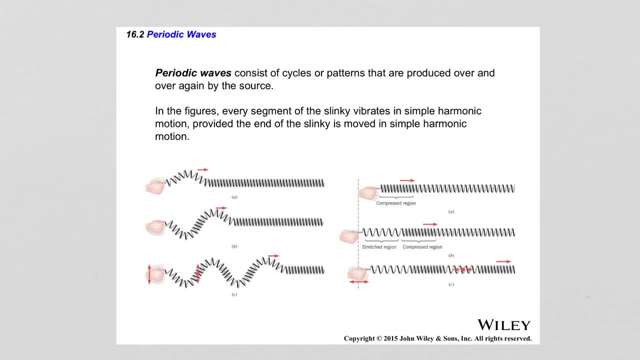 with equal periods of time between each disturbance. In this case, we have periodic waves created in the medium. Periodic waves consist of cycles or patterns that are produced over and over again by the source And, in the figures below, every segment of the slinky. 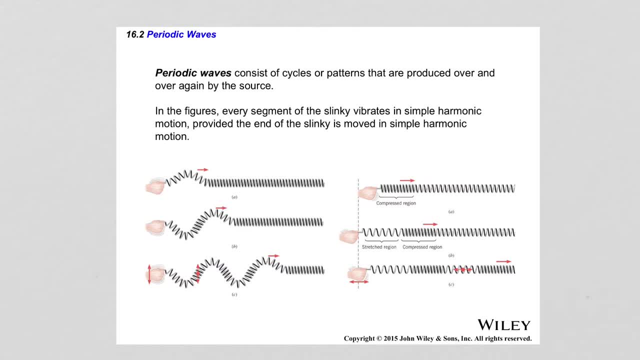 vibrates in simple harmonic motion And that means that the oscillations of the free end are not very large, are not with large amplitude. The oscillations of the slinky vibrates at the same speed and it takes the same amount of time for one full oscillation. 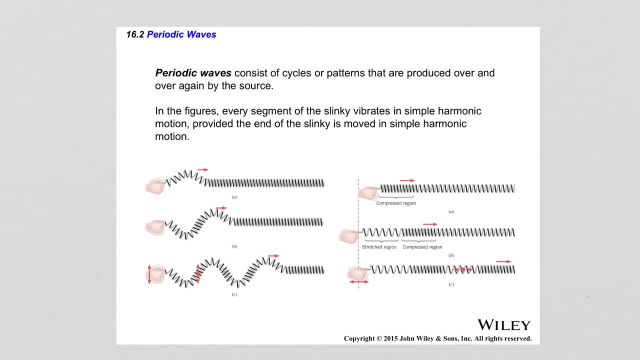 here of the source. to complete, If all these conditions are met, then the waves that are created in the slinky will be all exactly identical to each other. The same applies for a longitudinal wave, with the same amplitude every time, with the same speed every time. 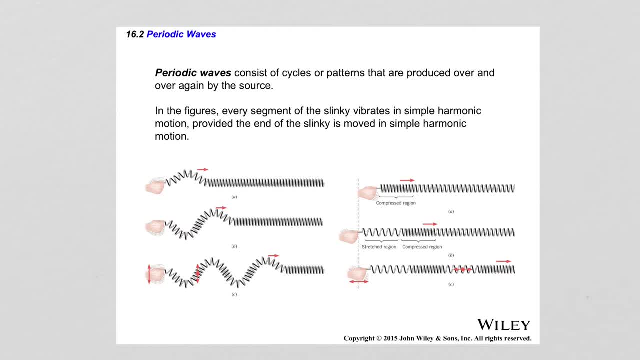 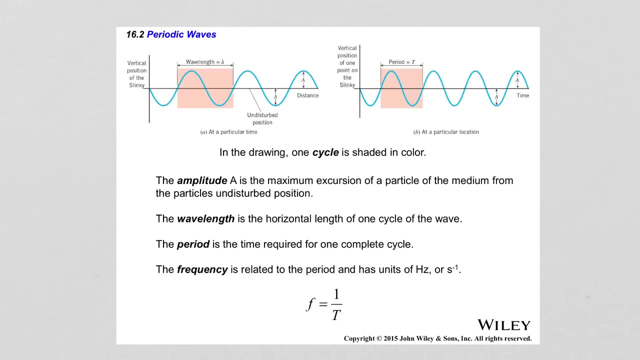 and it takes exactly the same amount of time to do one full oscillation. Then the series of waves created in the slinky will be all identical all the time, And so these series of identical waves created through a simple wave are defined through several quantities. 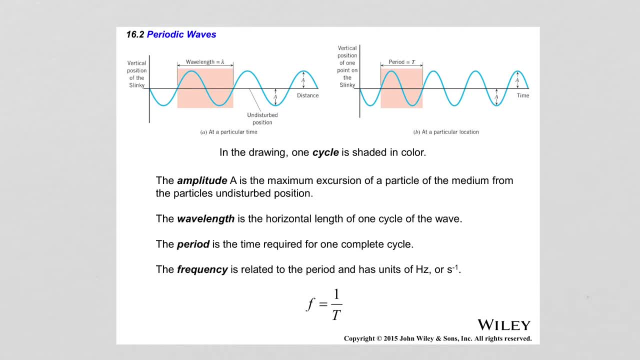 that we are going to talk about on this slide, And those quantities are amplitude, wavelength, period and frequency of the wave. To be able to define those quantities, it is useful to draw the waveform, in other words, a two dimensional coordinate system. 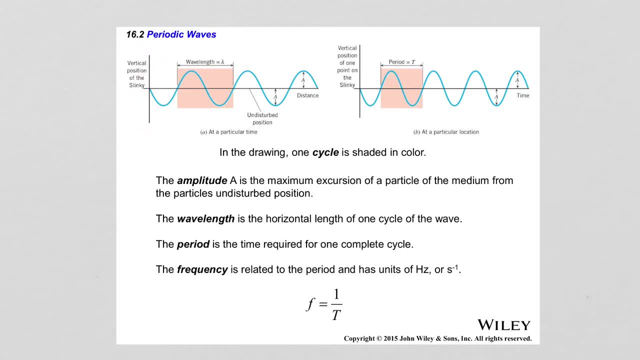 which consists of a vertical position, represented by the vertical axis, and then a spatial position, represented by the horizontal axis. So the amplitude of oscillations is the distance between the equilibrium position, so that is the horizontal axis position, and the furthest displacement from it. So 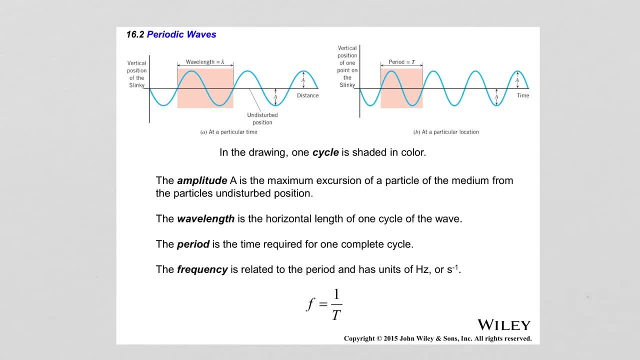 for this trough. here the amplitude is the distance from the horizontal axis to the bottom of the trough For this peak. here the amplitude is the vertical distance from the very peak of the wave to the horizontal axis. Now, as you can see the waveform that is shown here, 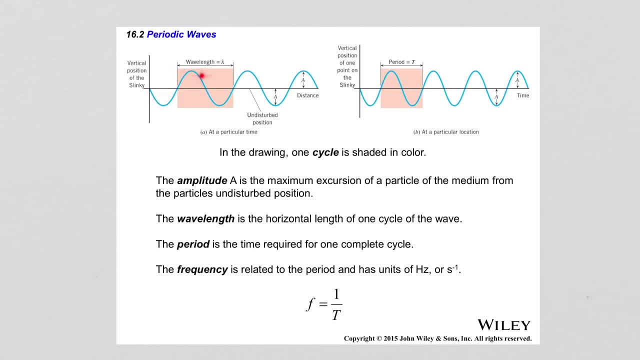 is cyclic, meaning the shape of the wave repeats after a certain amount of the waveform has passed. For example, if I start at the beginning of the coordinate system here, go down the waveform like, so when I get to this point, the next section of the waveform looks exactly the same. 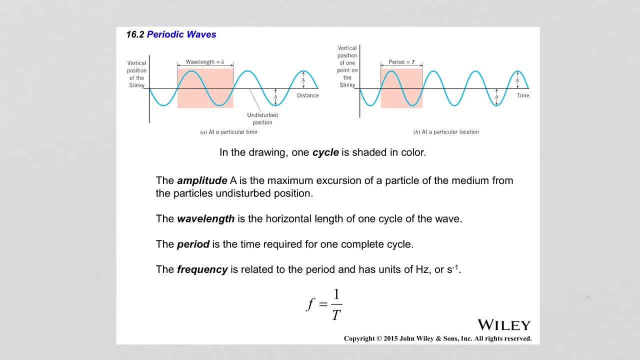 as the previous. So if I were to cut the waveform right here and here and superimpose the two sections on top of each other, they will be indistinguishable. They look exactly the same. I can't tell that they are two different ones. 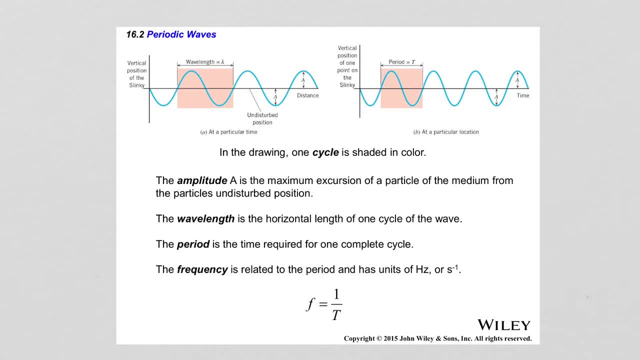 superimposed on top of each other, And so the distance along the horizontal axis, where I have a unique section of the waveform, is the wavelength of the wave. So here, for example, it is illustrated with a shaded rectangle and, starting from this point, going down the waveform, 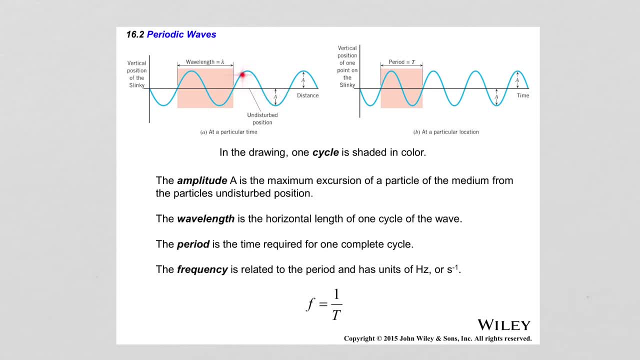 to this point. that is the wavelength of the wave. After that the shape repeats, so that is another wavelength of the wave. For example, it can be from here to here. That is also the wavelength, So let's label that And then, using this, 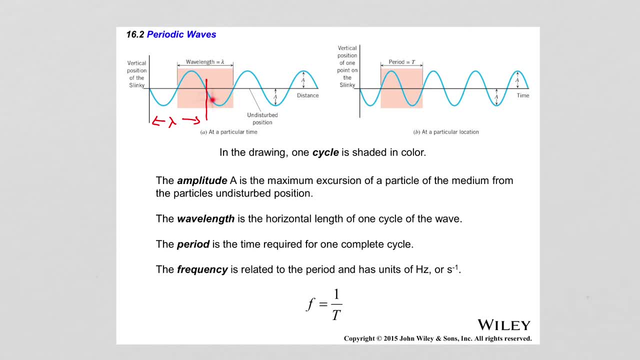 as my reference pattern, starting from this point, moving down the waveform that is another wavelength of the wave, And so on and so forth. So there is now a set rule where you start to measure the wavelength of the wave. as long as you adhere to the rule that 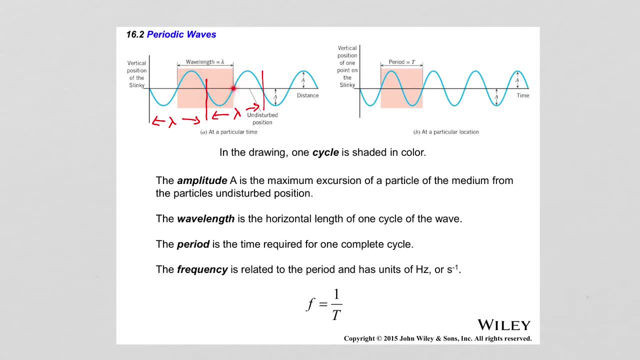 you go down the waveform until you reach a point after which the waveform repeats itself. So every unique region of the waveform is the wavelength. The wavelength is labeled with the Greek letter lambda. Another important property for describing waves is the period of oscillations. 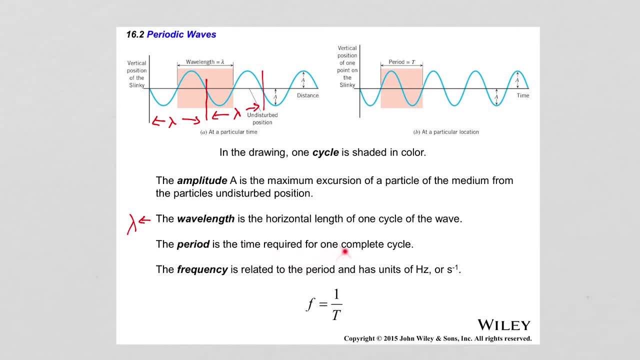 The period is defined as the time required for one complete cycle. In this graph here we have the waveform of the wave shown again. The vertical axis indicates the vertical position of a point in the medium And the horizontal axis represents time in this case. 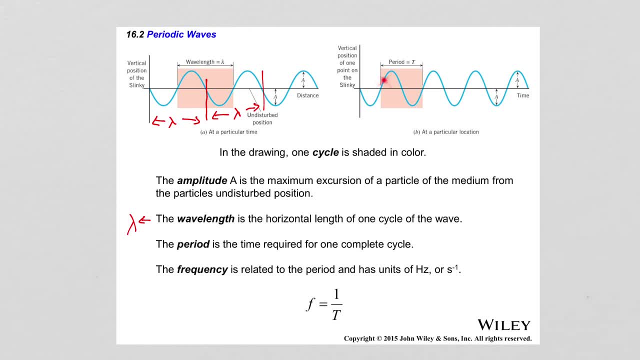 So one unique section of the waveform takes the amount of time that is known as the period of oscillation. The section after this unique section repeats the waveform pattern. The next section to complete is also the period of the wave. Again, the period can be measured. 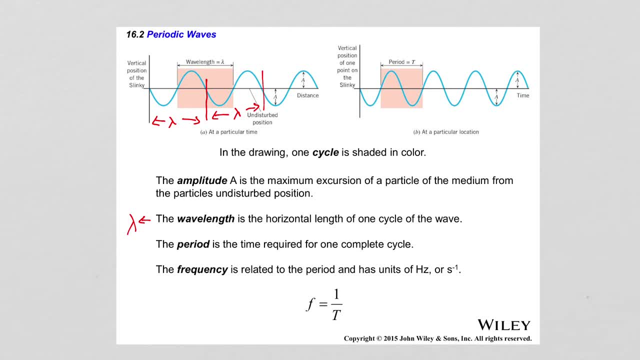 from different starting points. on the waveform, For example, I can start at the trough here and go to the next trough, So the time it takes to get from this position to this position is also the period of the wave. I can also do the same. 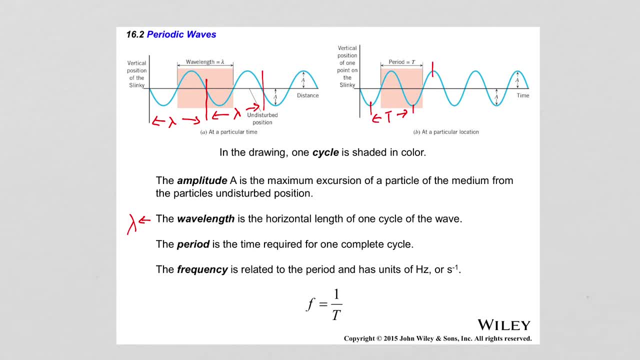 here and go down the waveform, get to the next peak. The time it takes to get between those two points is also the period of the wave. So as long as you observe the important rule about how you identify unique sections of the waveform, you will be able to. 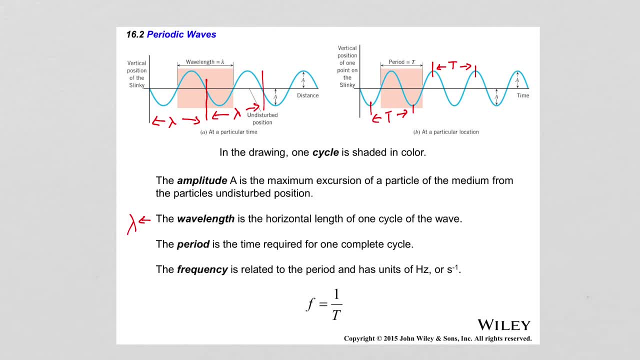 determine the wavelength of a wave. The period is labeled with capital T And typical units for the period are seconds. typical units for wavelength are meters. However, denominations are also possible depending on the type of wave in consideration. The last quantity I want to discuss. 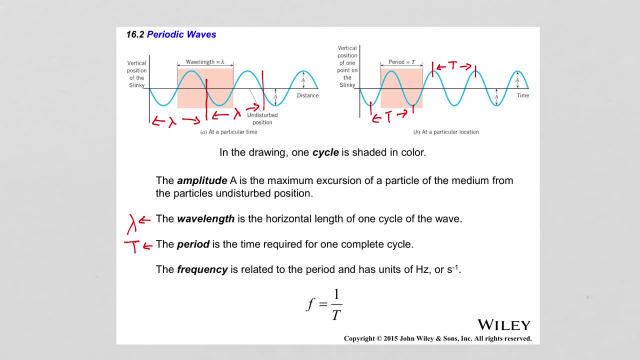 in relation to describing the properties of waves is the frequency of oscillations. So the frequency is related to the period, and the formula that relates the two quantities is that the frequency is equal to one divided by the period, So it's proportional to the inverse of the period. 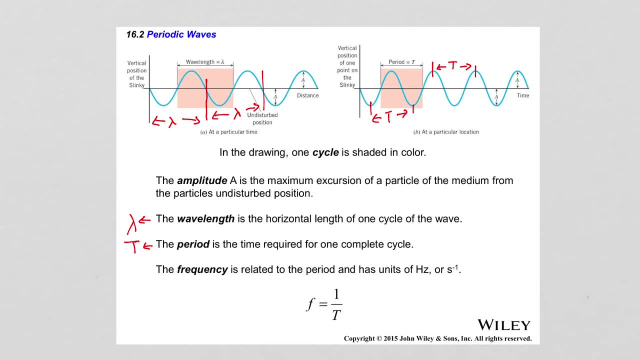 The units for frequency are in terms of the periods or in terms of the units of the periods. that is inverse. second, So how do we define frequency? if you look at the waveform? So let's look at the waveform right here. Or rather, let's look at the waveform. 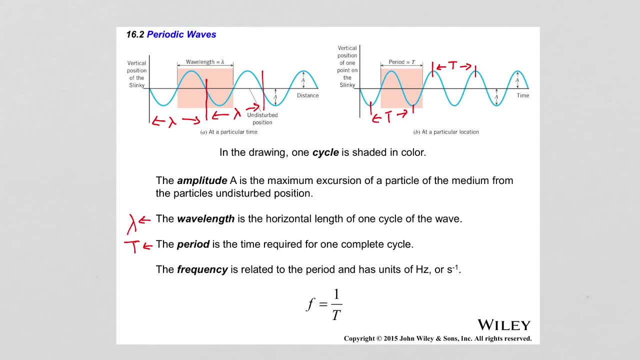 right here on the right graph. So the frequency is the number of oscillations per second, so the number of oscillations of the waveform per second. So what does that mean? It means how many complete cycles pass through a point in space in one second. 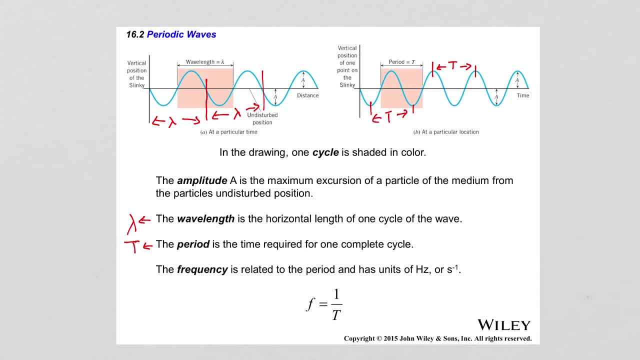 That is the frequency. So for example, if we have one complete cycle of the waveform passing through a point in space, then that would be a frequency of one hertz. If we have two complete cycles passing through a point in the medium in one second, that would be. 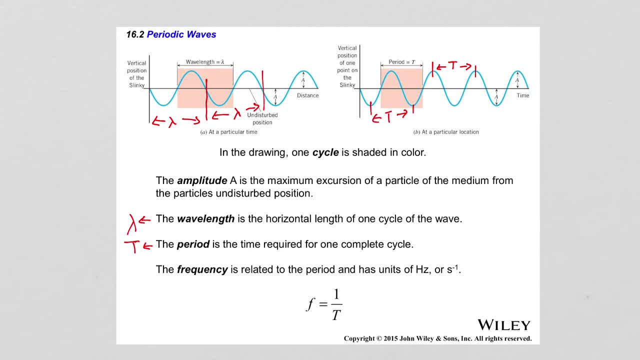 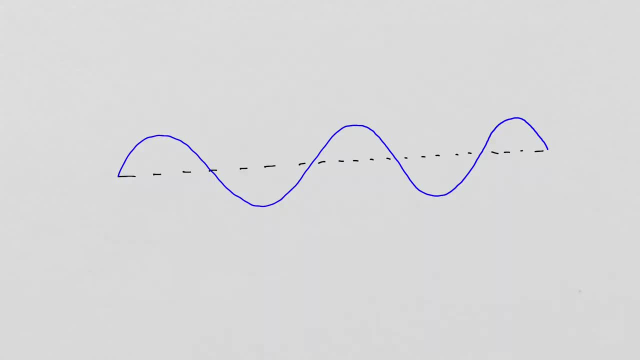 a frequency of two hertz. If we have fifty complete cycles passing through a point in the medium in one second, that would be fifty hertz, and so on and so forth. Let's consider a periodic wave that is created in a rope, So we have a pattern of 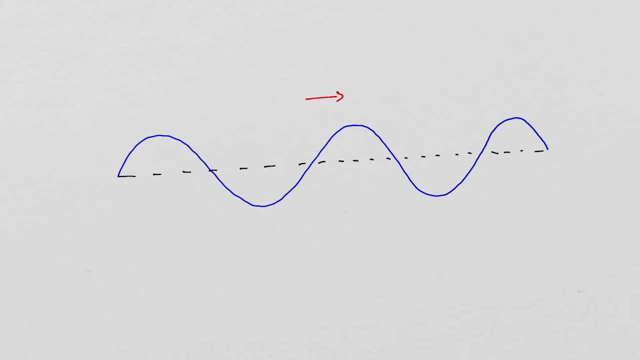 oscillations that move away from the source of the disturbance. let's say the source is right here at the free end, oscillating up and down, and so the wave pattern moves away from the source of the disturbance with some velocity v. We discussed two important parameters. 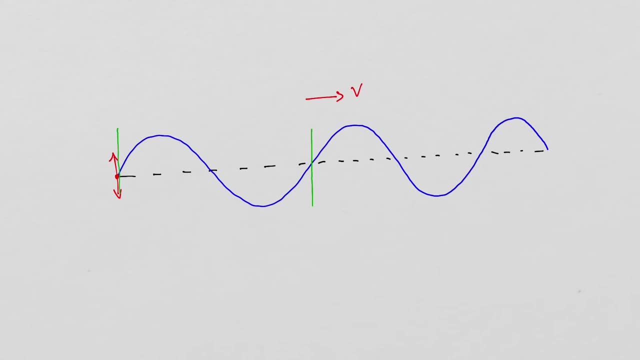 of the wave and those were the time between those two points. for example, We also discussed the period, and that is also the time, for a unique segment of the wave front to pass through a certain point in the medium. So the time for one full wavelength. 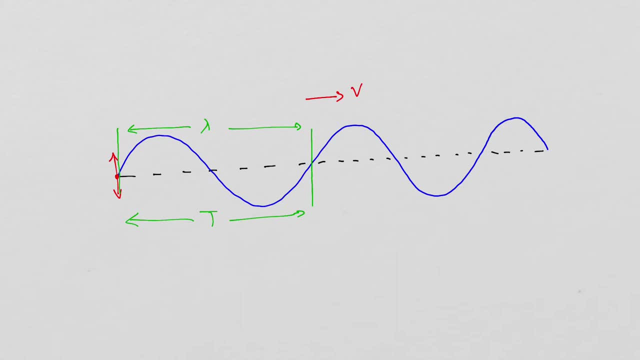 so there has to be a relationship between the speed of propagation of the wave in the medium, the wavelength of the wave and the period of the wave. and this relationship is very simple: the speed is equal to the wavelength divided by the time. to give you an analogy with 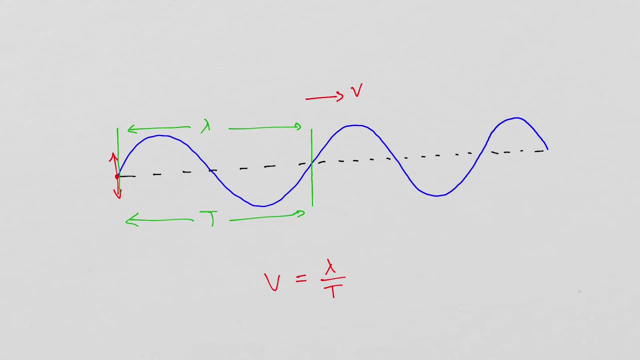 a simple concept such as linear motion, even though this is a completely different concept, meaning the waves are a completely different concept compared to linear motion. you can still think of this formula here as distance divided by time, because wavelength is simply the length of wave that passes through. 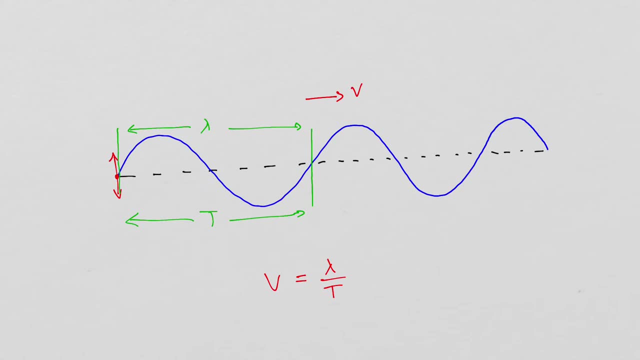 a point in space, in the time, which is the period of the wave. so wavelength divided by time is the speed of the wave, wave speed. there is also a relationship, as we discussed on the previous slide, between the frequency of the wave and the period. so we know that the frequency 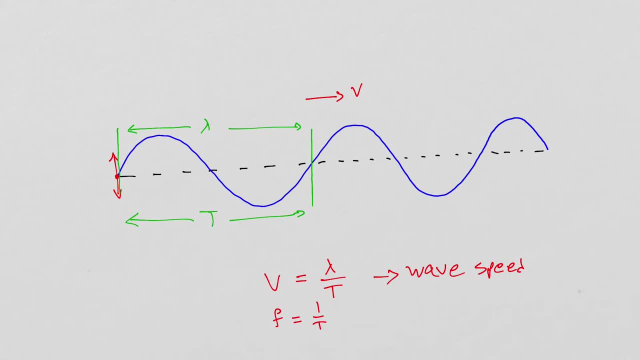 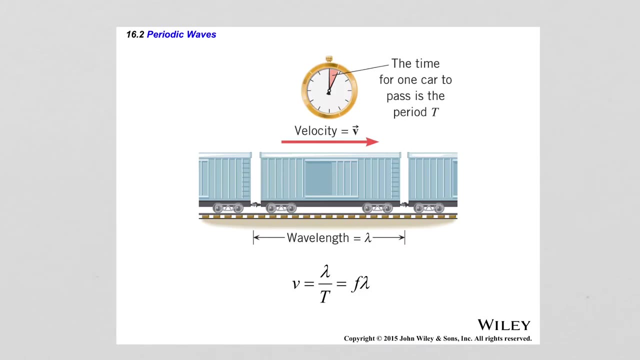 is equal to the inverse of the period. so if I combine the two, I end up with a very important relationship between the speed of propagation of the wave, the frequency of the wave and the wavelength of the wave. this relationship we are going to use often, and so the speed 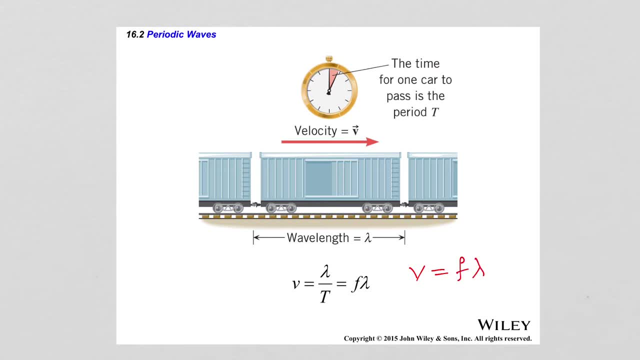 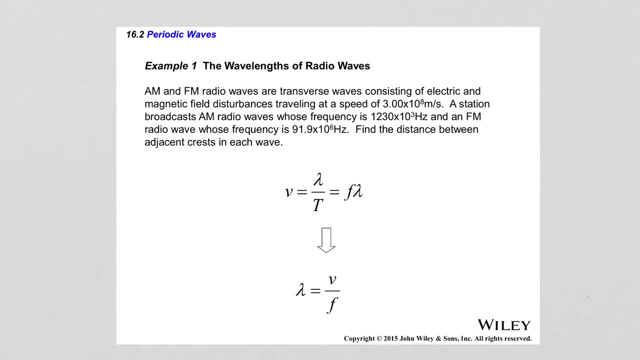 of the wave is equal to the product of the frequency and the wavelength of the wave. the relationship between the speed of the wave, the frequency and the wavelength of the wave is very useful in determining the wavelengths or the frequencies or speeds of various waves. for example, there are two types of radio waves. 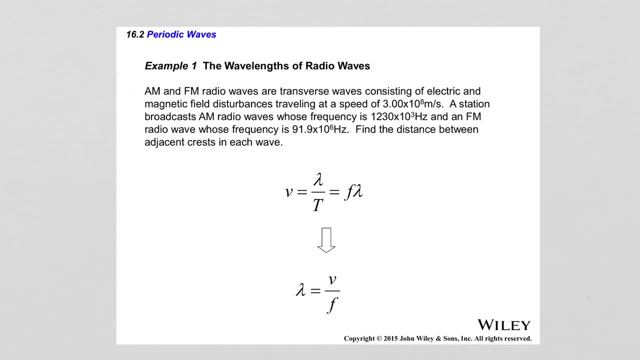 there is AM and FM radio waves. if you listen to a radio, the more common frequency which is used is FM. however, of course you can tune your stations to some AM frequencies. usually you get more interference with those. there is lots of noise, and all that with FM frequencies. 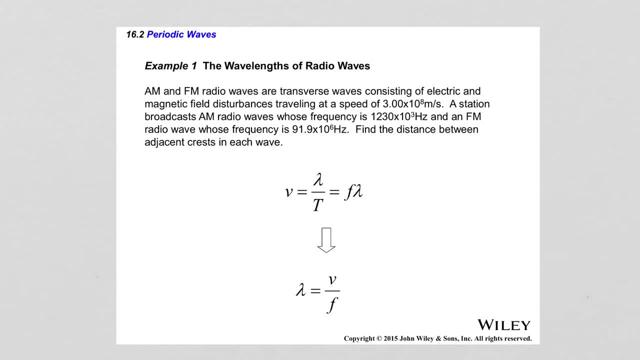 the sound is very clear and easy to listen to. so AM and FM radio waves are transverse waves. as I described at the beginning of the presentation, they consist of electric and magnetic field disturbances, so we do not need to know exactly what these disturbances are and how they work. 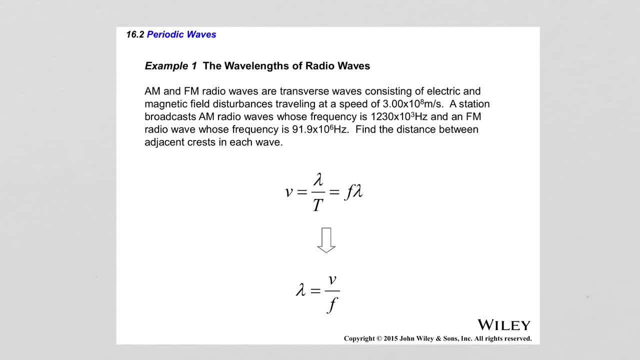 and why they are caused by such disturbances. and since AM and FM radio waves are part of the electromagnetic spectrum and light is part of that as well, we know that the speed of propagation of those waves is equal to the speed of light, and that is 3 times 10 to the 8 meters per second. 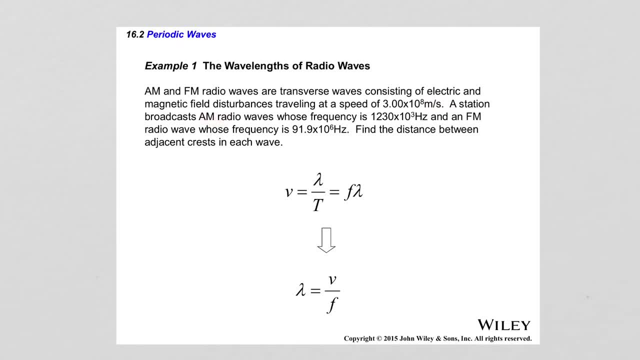 so a station broadcasts AM radio waves with frequency of 31.9 times 10 to the 3rd hertz and FM radio waves with frequency of 91.9 times 10 to the 6th hertz. the question is: what is the wavelength? 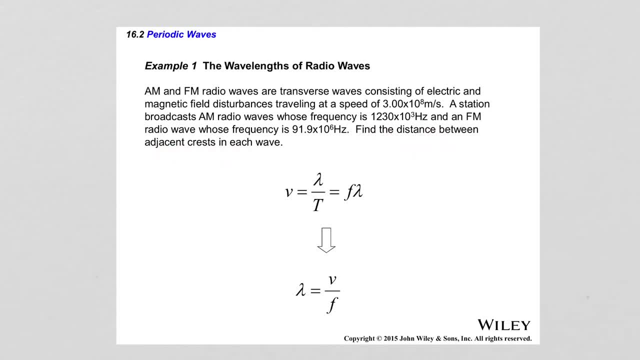 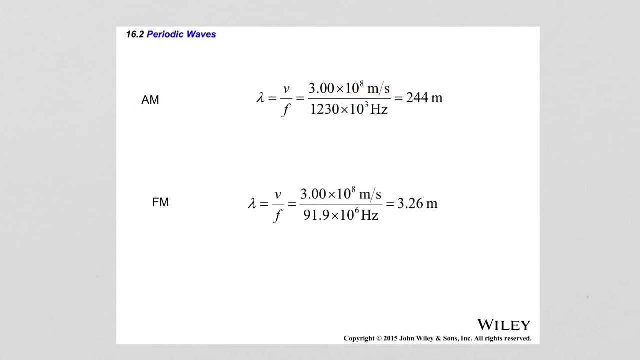 of those two waves. so starting with the relationship that the speed is equal to frequency times wavelength, so that is the ratio of speed and the frequency. and so for the AM radio waves we have 3 times 10 to the 8 meters per second, divided by 1230 times 10 to the 3rd hertz. 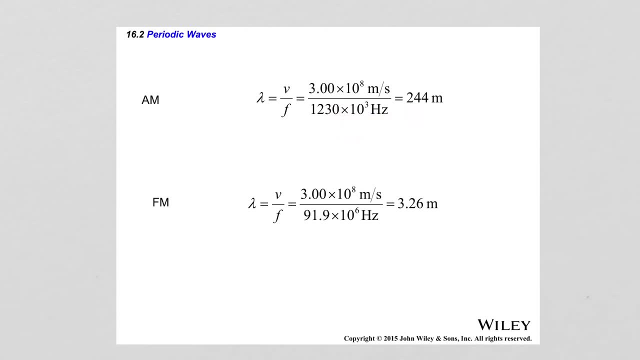 that is 244 meters. for FM frequencies we have 3 times 10 to the 8 meters per second, divided by 91.9 times 10 to the 6th hertz, or that is 3.26 meters. so if you read the wavelengths, 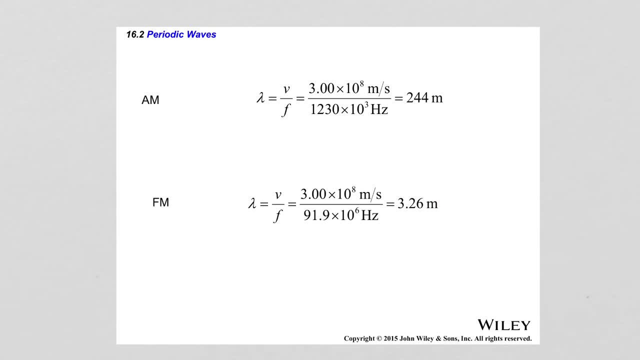 for those two waves you can and compare them. you can understand why radio broadcast with AM frequencies has so much noise in it. these wavelengths are very, very long, so 244 meters is more than 700 feet long wavelength. so there is plenty of um. let's say 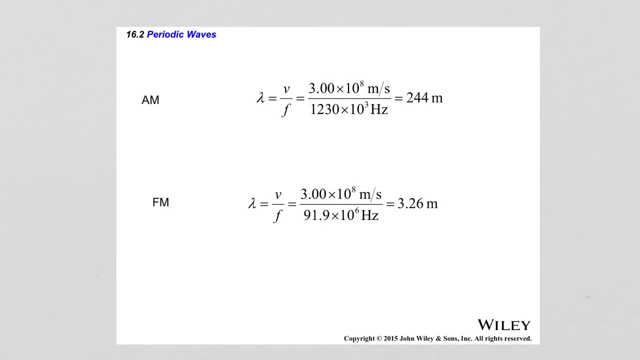 for interference from other waves or sources to sort of contaminate the broadcast. and then you get this um um noise effect when you listen to AM stations. compared to FM radio waves, which are very short, there is very little possibility for um the broadcast at FM frequencies. 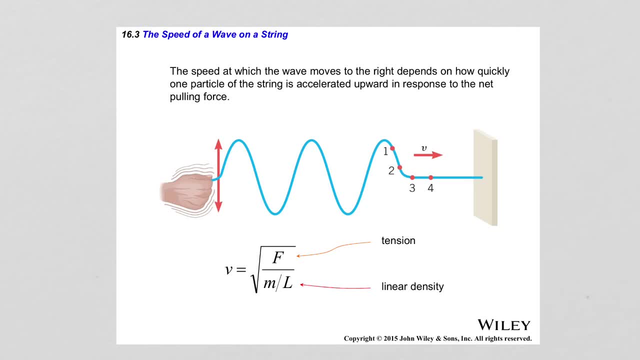 are much cleaner and um with very little noise. in the previous slides I defined the speed of wave propagation based on the characteristics of the wave itself. however, the speed of propagation also is determined by the physical properties of the medium. so the speed at which the wave moves. 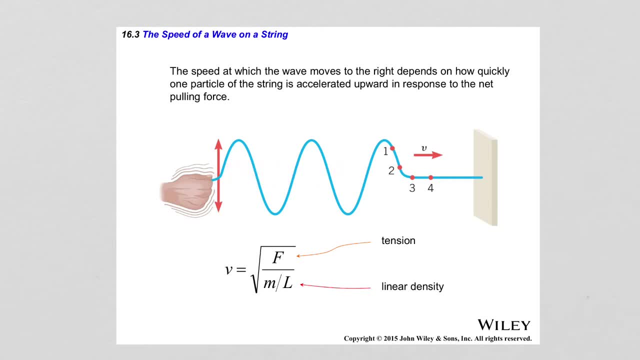 to the right in this rope depends on how quickly one particle of the string is accelerated upward in response to the net pulling force, and the net pulling force is the force generated along the rope by the adjacent particles in the rope, and so it turns out that the speed of propagation. 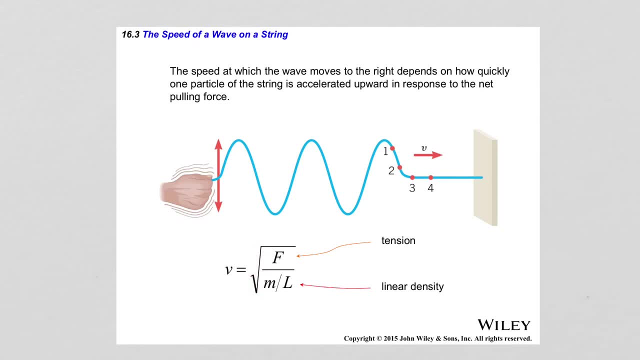 is equal to the square root of the tension in the rope divided by the ratio of mass to length. for the rope this ratio is called linear density or also linear mass density. so that is the mass of the rope divided by the length of the rope. notice that. 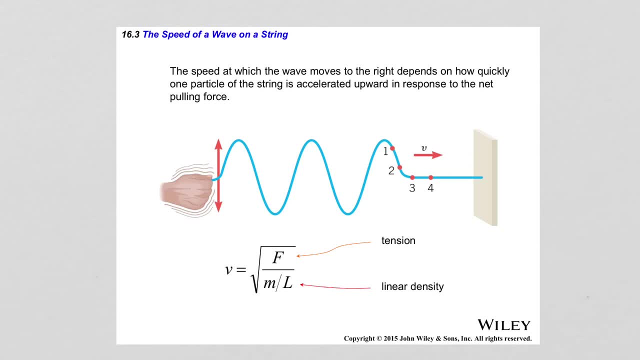 for a um uniform rope or string or cable, where there is no mass or density variations along the rope, the ratio of mass to length is a constant. so for any length of the rope if you know the mass then you are going to get the linear mass density for that rope. 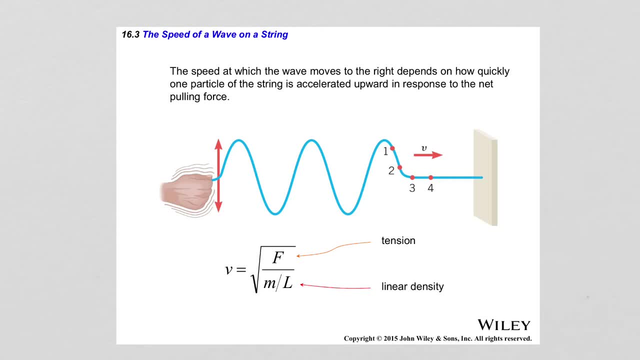 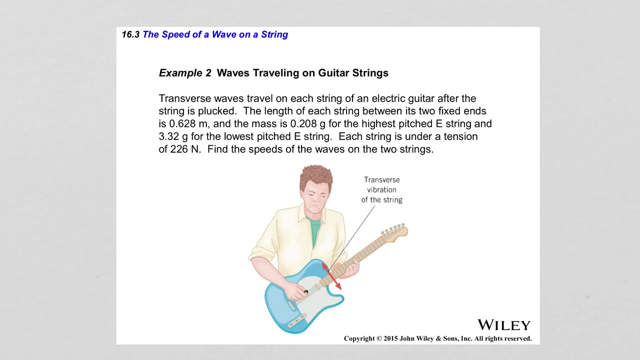 and so again. the speed of propagation is a function of the properties of the medium. is for um ropes or for solids in general, is the tension divided by the linear mass density? here is an example that illustrates that concept. so let's find out the speed of propagation. 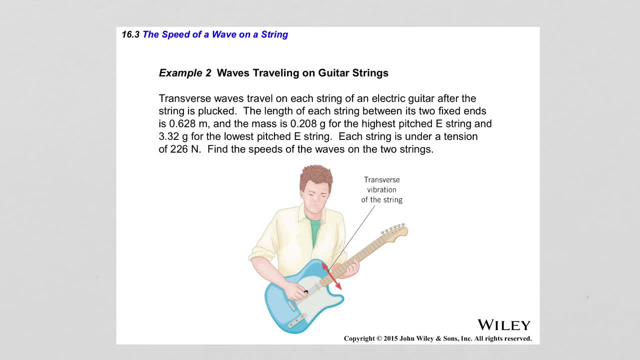 of the rope, so let's take a look at the speed of propagation of the rope. so let's take a look at the speed of propagation of the rope. let's take a look at the speed of the rope of the rope, so let's see how the speed 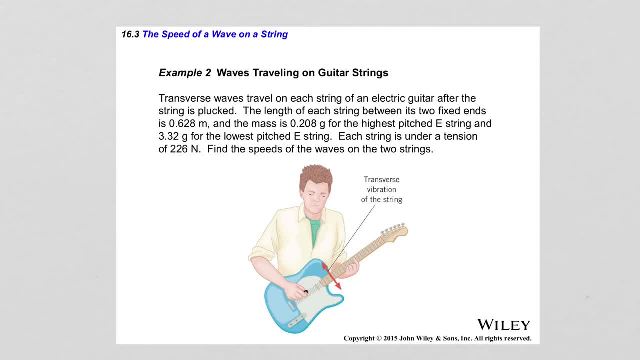 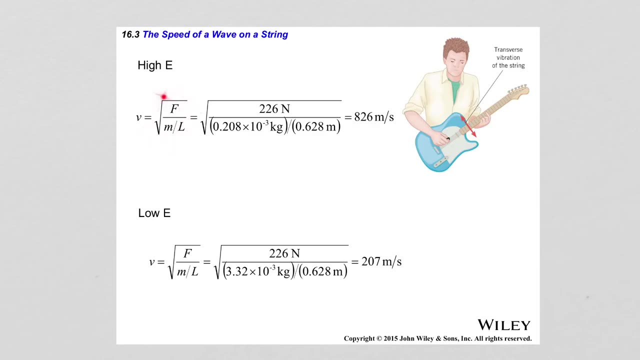 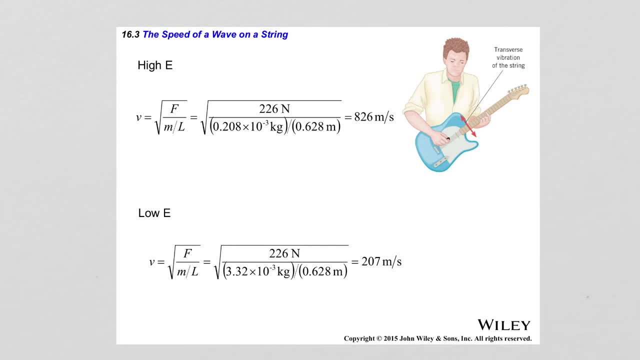 the mass is converting kilograms divided by the length, which is 0.628 meters, that gives us 826 meters per second, and for the low E string, the value for the speed is 207 meters per second. you can see how, in the lighter string, the speed is. 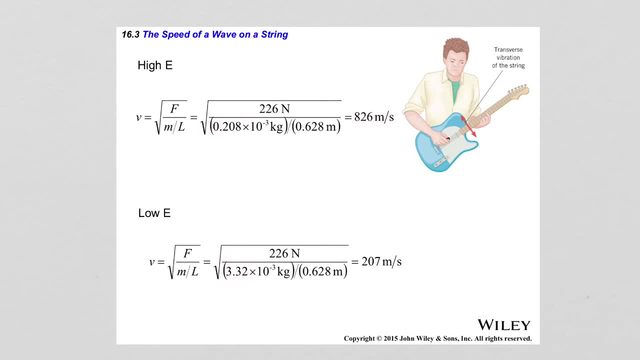 much higher compared to the heavier string. you can also relate this to the pitch that you hear when those two strings are plucked. the high E will have high pitch, or in other words, higher frequency, and the low E will have low pitch, or in other words, lower frequency. 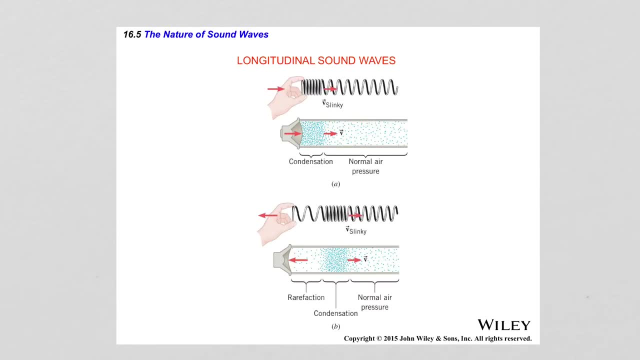 let's now discuss the nature of sound waves. sound waves are longitudinal waves and I introduced longitudinal waves by using the model with a slinky. we're pushing back and forth causes creation of compressions and rarefactions, or stretching stretched regions in the slinky, and so repeating that process multiple times creates a periodic wave in the. 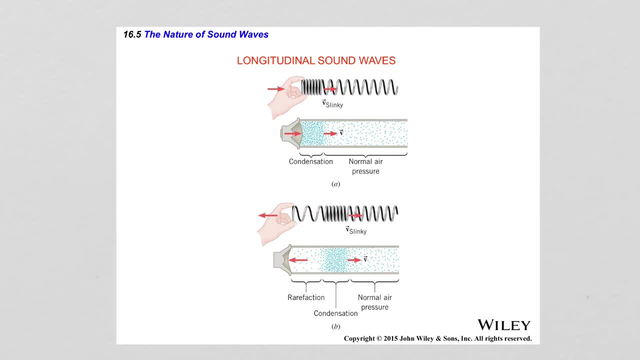 slinky. now let's see how this works with sound waves propagating in gas. consider a loud speaker that is attached to one end of a tube that's filled with air. so when a sound note is played through, the loudspeaker membrane here vibrates back and forth. So when the membrane moves to the right, it comes in. 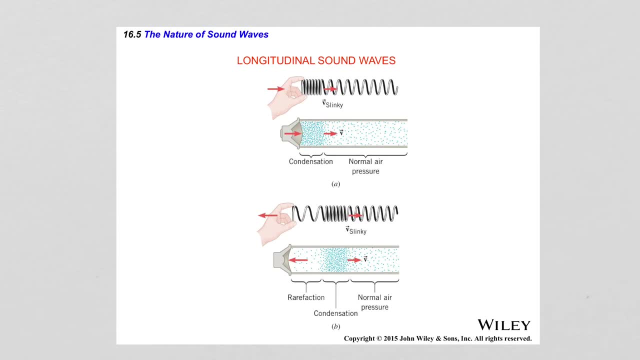 contact with the air molecules that are closer to it and physically moves them to the right as well, with some velocity V. The result of this process here is a creation of a higher density region of the gas, which we will call condensation. The rest of the air here is with normal concentration of 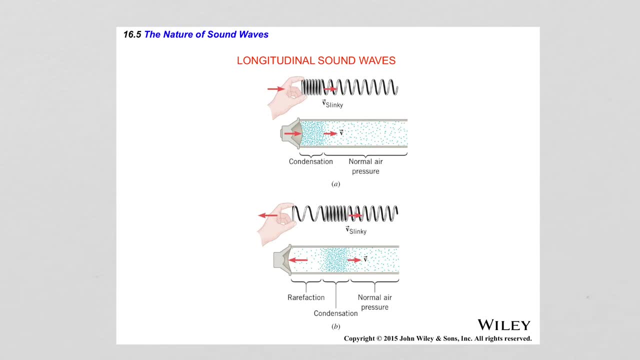 molecules per unit volume. Then the membrane moves backwards, which creates a smaller density region with the molecules of the gas. Then the membrane moves backwards, which creates a smaller density region with molecules of the gas. We're going to call that rarefaction. And so now we have two distinct regions: one with higher density of 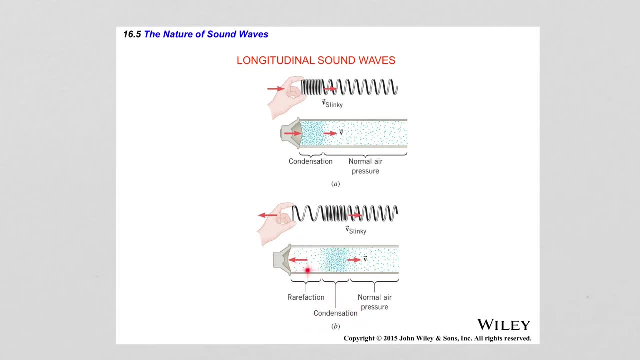 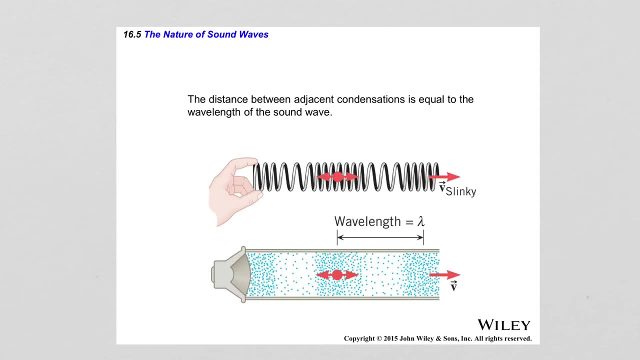 molecules, that's the condensation, and one with smaller density of the molecules, that's the rarefaction. Now, repeating this process, the membrane, going back and forth multiple times, will result in the creation of multiple condensation regions and multiple rarefaction regions. So then one could: 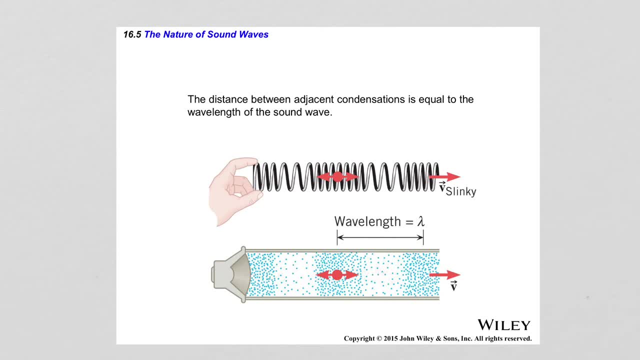 measure the wavelength of the sound wave created in the gas here by taking a unique portion of the created wave, such as, for example, from the middle of this condensation to the middle of the previous condensation. so that would be the wavelength of this sound wave And, of course, the time that it takes for one. 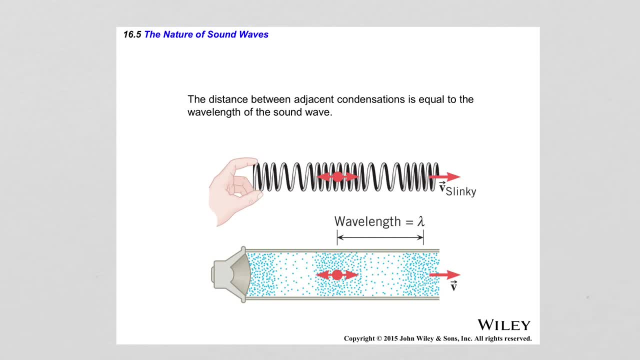 for wavelength to pass through a region in the gas, that would be the period of the wave, And once we know the period we can also calculate the frequency of the sound wave in here. One important remark here is that the gas molecules do not move like the sound wave. 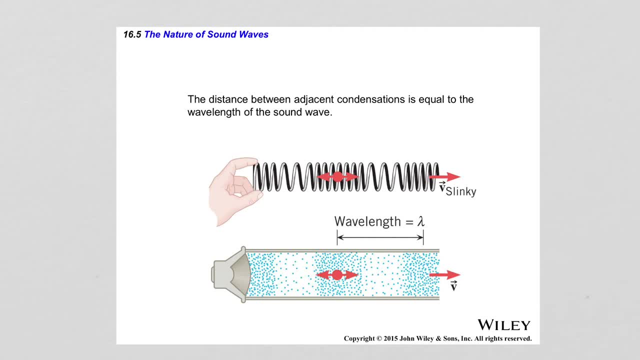 away from the membrane of the loudspeaker as the sound is played. As the membrane moves back and forth, the molecules also move back and forth. The sound waves actually transfer through or propagate through the gas, by the molecules in the gas interacting with each other. 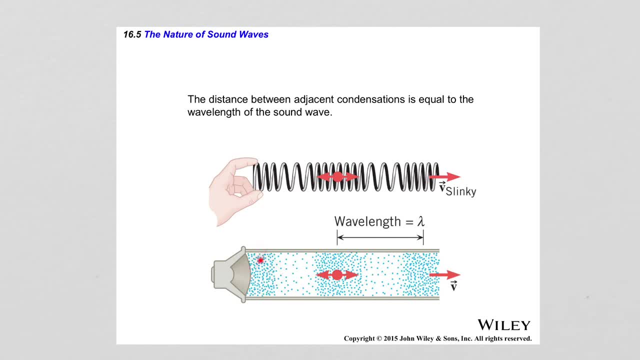 So the higher density of molecules here causes these molecules to interact with each other more, And so, as a result, the momentum of the molecules changes as the molecules that are closer to the membrane hit the molecules or collide with the molecules that are next to them. 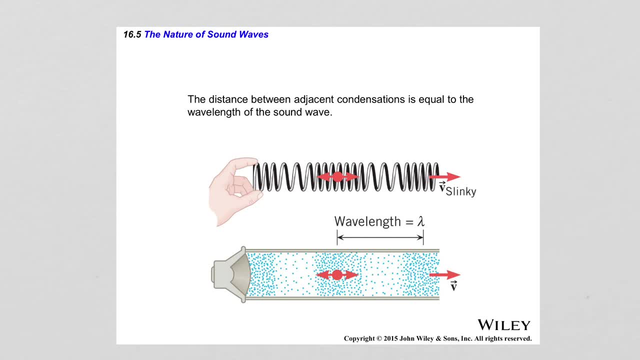 Those molecules collide with the molecules that are after that, and so on and so forth, And so, as the condensation here is formed, the molecules that are closer to the membrane as the membran- starts to move the other way now are free to move in opposite direction. And 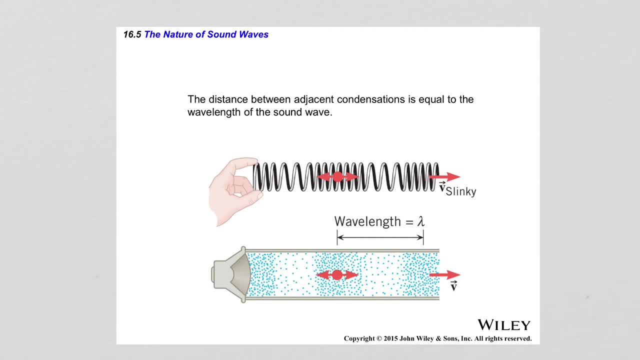 so if enough molecules move in the opposite direction, a rare fraction is created. In the meantime, the molecules from the condensation have interacted with the molecules in the gas after them, so the condensation effectively has moved further away from the membrane, And so we have a constant motion of the. 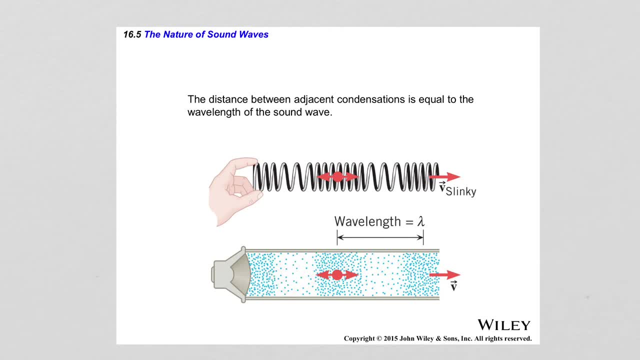 molecules back and forth in the entire gas, but we also have these higher concentrations of molecules and those lower concentrations of molecules alternating and going away from the membrane. So similarly to the model of the particles in the rope moving vertically up and down but actually not. 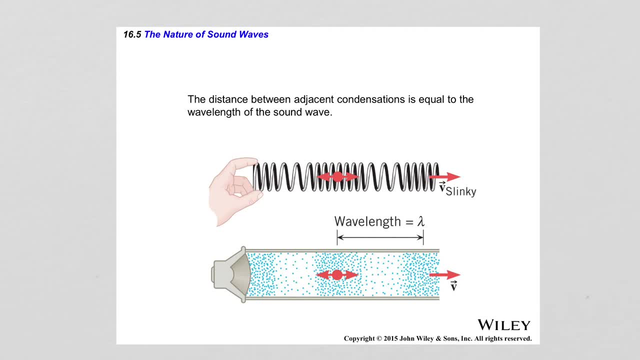 moving in the reverse direction, away from the source. only the wave moves through the medium. Here we have motion of the molecules moving left and right, only the waves created in the gas. so the condensations and rarefactions are moving away from the source. 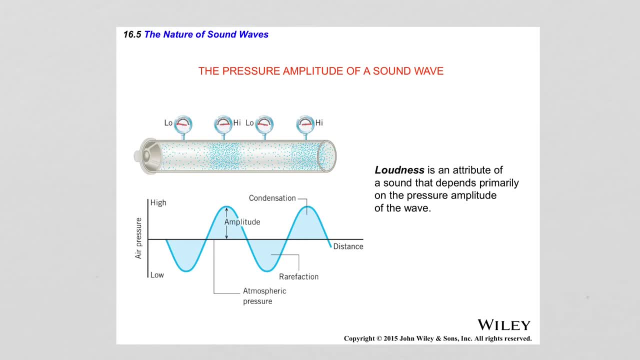 Another important quality of sound waves is the loudness of the wave. That is an attribute of sound that depends primarily on the pressure amplitude of the wave. So what is the pressure amplitude? When I explained the creation of condensations and rarefactions, I talked about the gas. 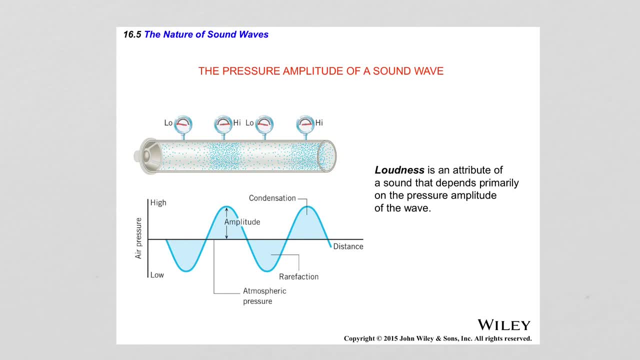 molecules in the condensation have higher density than the gas molecules in a rarefaction. Or in other words, that translates to high pressure of the gas where we have a condensation And lower pressure in the gas where we have a rarefaction. So if there was a way to measure the pressure in a gas when a sound wave is, 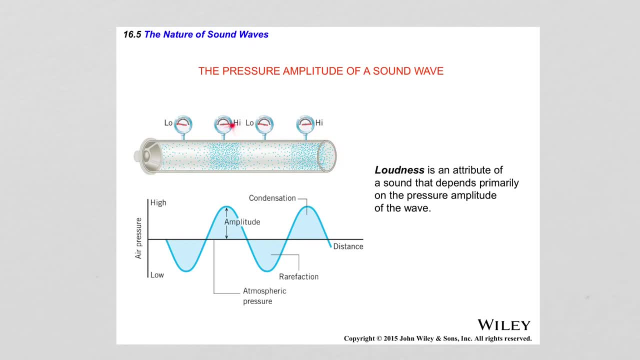 created in that gas. for example, as shown here, we'll measure low pressures where the rarefactions are and high pressures where the condensations are, And so these pressures can be translated into amplitude of air pressure. So if we plot air pressure versus distance for the gas, we are going to end up with a. 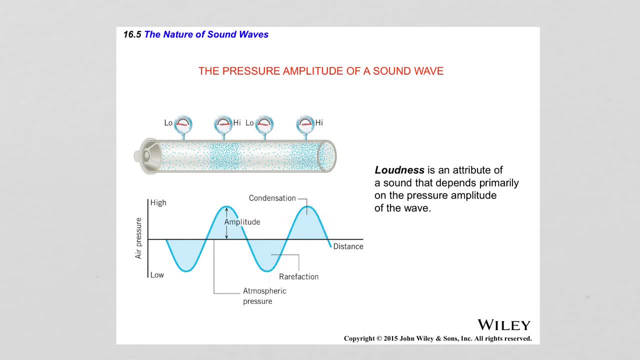 periodic function that will have amplitude equal to the pressure in the condensations or rarefactions, and also periodic behavior, just like any wave. So the higher the amplitude, the louder the sound. The lower the amplitude, the quieter the sound. To illustrate the idea how the pressure of the gas corresponds to the loudness of the sound: 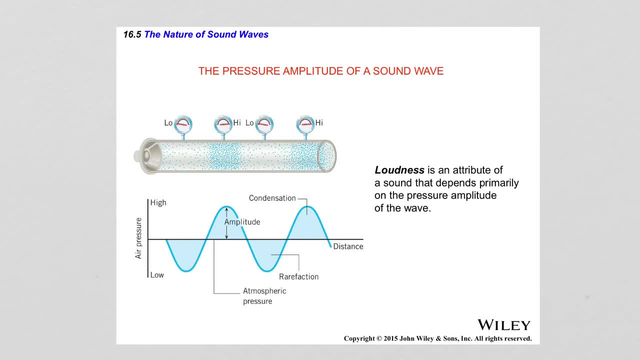 think about it this way: You're pronouncing a sound with your regular tone of voice, and that sound will come out of your mouth with certain loudness. Now shout out that same sound. Obviously, the loudness will be much higher, and that is because 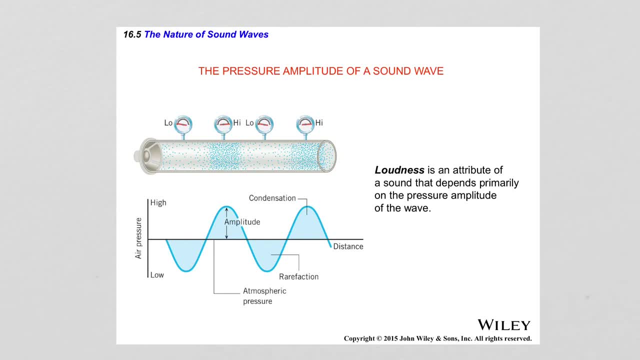 you created a lot more pressure when you were pronouncing the sound compared to when you're using your normal voice, And so the pressure amplitude between the two cases- the difference in the pressure amplitudes between the two cases- is significant. As a result, the loudness of the 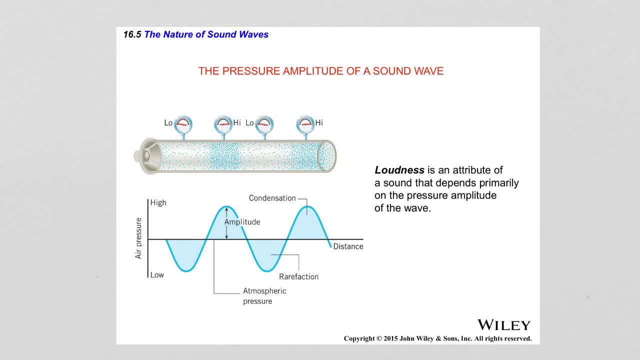 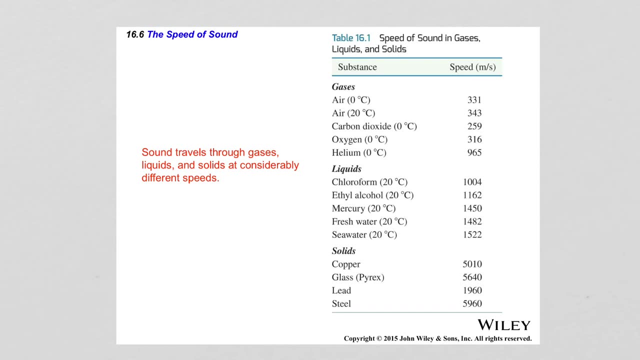 sound also is significant. The difference in loudness of the sounds is also significant. The speed of sound depends on the material in which the sound propagates and also on the temperature in the medium. So for gases the speed of sound is the lowest compared to liquids and solids, And for liquids the speed of sound is higher. 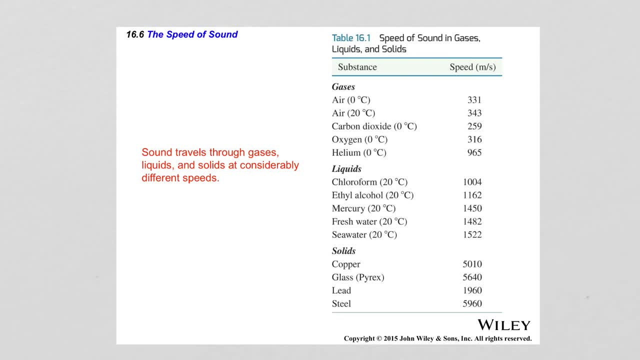 than gases, but lower than solids. In solids, the speed of sound is the highest. This is purely due to the physical structure of those media. For gases, the molecules are spread further apart from each other, so it takes much longer time for molecules to interact with each other, which 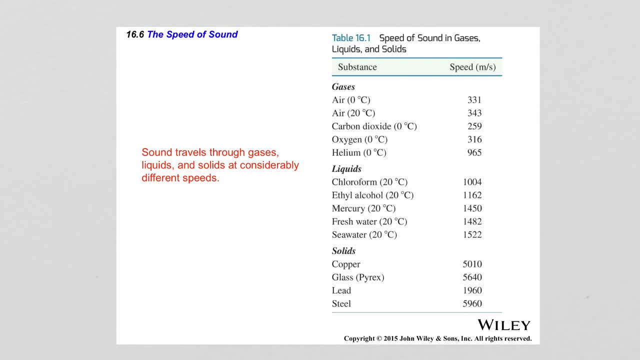 then translates into slower propagation of the sound waves. In liquids, the molecules are much closer to each other, which means that the times of interaction between the molecules are much slower, which results in higher speeds of propagation. And in solids, atoms or molecules are packed very close to each other, which decreases the time of interaction. 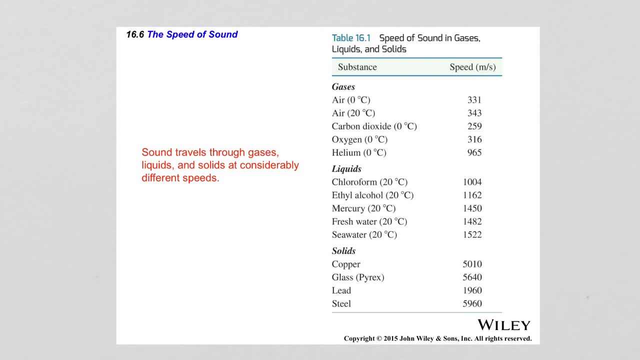 significantly, which increases the speed of propagation also significantly. The second point was that the speed of sound depends on temperature. For example, for air at zero degrees celsius the speed of sound is 331 meters per second, but at 20 degrees celsius we have 343 meters per second. In problems where the speed of sound in air is not specified directly. 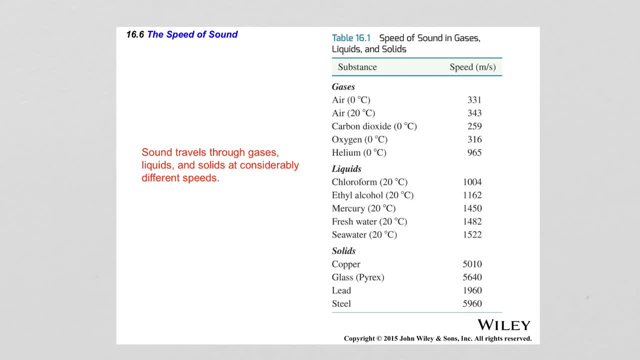 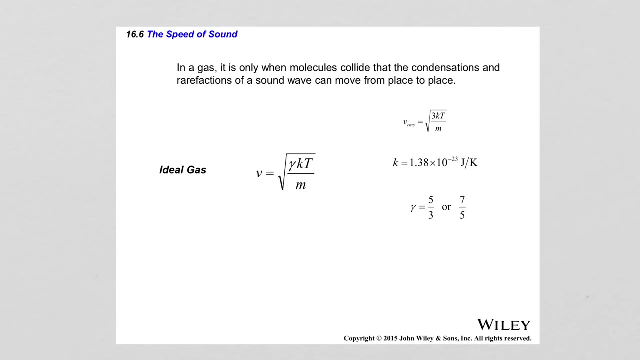 but it's uh, it's needed to be used for calculations. we will always assume that the speed is the speed of sound in air at 20 degrees celsius, which is 343 meters per second. The speed of sound can be calculated purely from the wave properties. 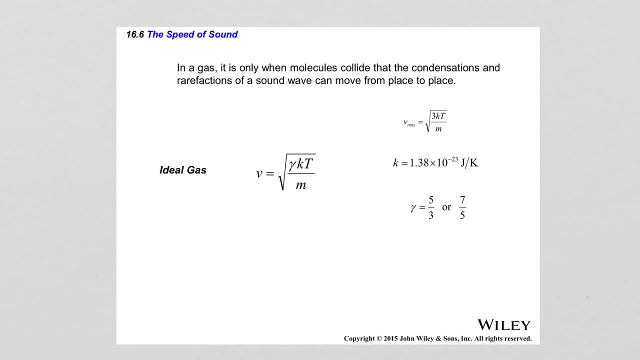 as wavelength and frequency or period. However, the speed of sound in gases can be also calculated in terms of the physical properties of the medium in which the wave is propagating. A formula that can calculate the speed of sound in gases is shown here. 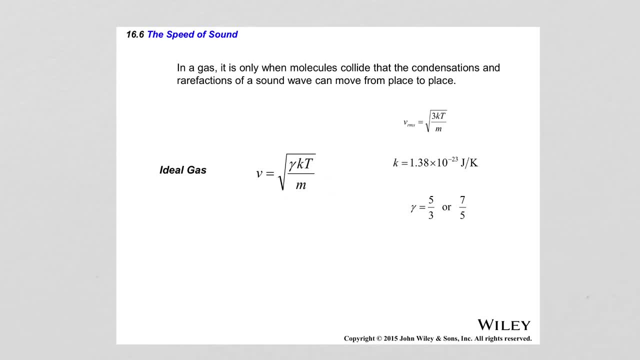 This is the speed of sound in what we call ideal gas. Ideal gas is a theoretical gas composed of many randomly moving point particles that are not subject to inter-particle interactions, Or in other words, the gas is placed in such a large volume that the molecules rarely interact. 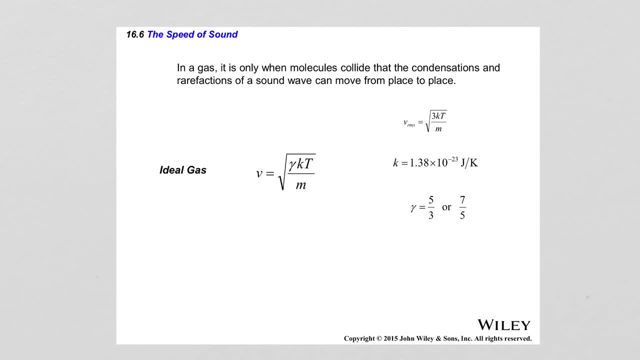 with each other, if at all. So in that model, the speed of sound is calculated as the square root of this coefficient gamma, which can take two different values: five-thirds or seven-fifths, Where five-thirds is used when we are dealing with mono-atomic gas, and seven-fifths is used 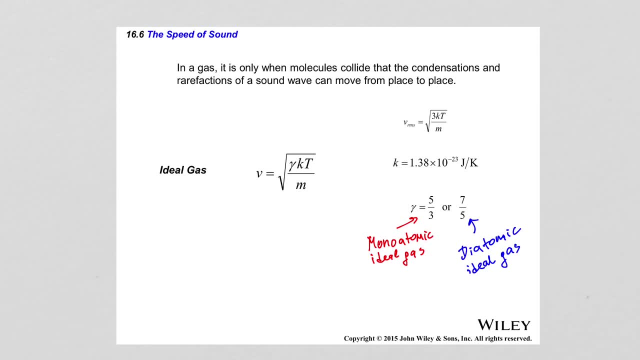 when we're dealing with diatomic gas. K is the Boltzmann constant, which is equal to 1.38 times 10, to the negative 23rd joules per kelvin times, the temperature of the gas in kelvin divided by the molar mass of the gas, molecular mass of the gas, rather. 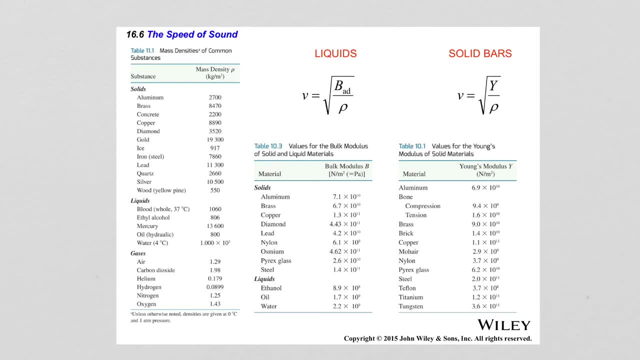 Similarly, the speed of sound can be calculated for liquids and solid bars using the following two formulas. For liquids, the speed of sound can be calculated for liquids and solid bars using the following two formulas: The speed of sound is equal to the square root of the bulk modulus divided by the density of the liquid. 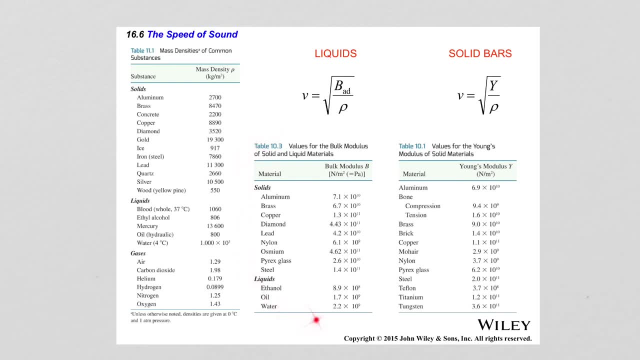 And the bulk modulus is a table quantity. For example, some of the values for different materials are presented in table 10-3.. And for solid bars, the speed of sound is calculated as the square root of the young modulus divided by the density of the material. The young modulus is also a table quantity, which is 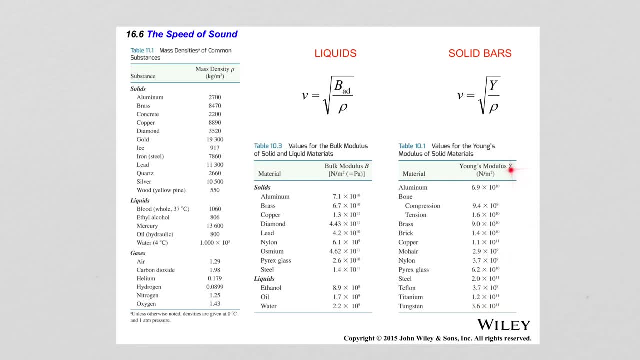 some of the values of it, which are shown in table 10.1.. So, to reiterate, we have two ways of calculating the speed of sound in different materials. One is through the properties of the waves, such as wavelengths, frequencies and periods. 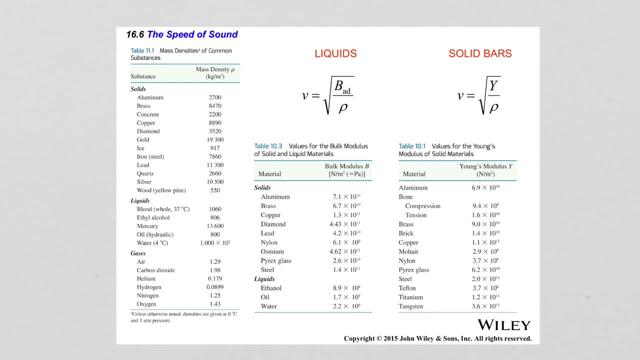 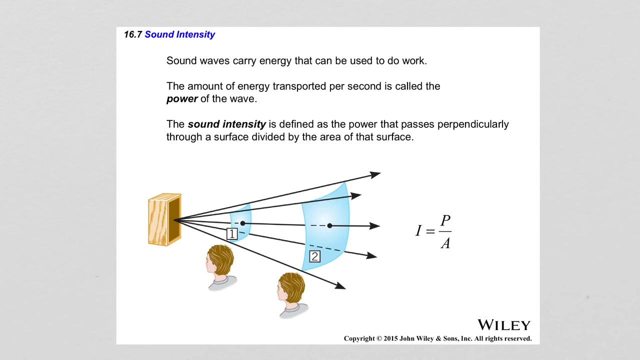 and the other is through the formulas involving the bulk modules, the young modules, and also, for ideal gas, the Boltzmann constant, the temperature of the gas and the molecular mass of the gas. When I started the lecture, I said that all waves have two main characteristics. 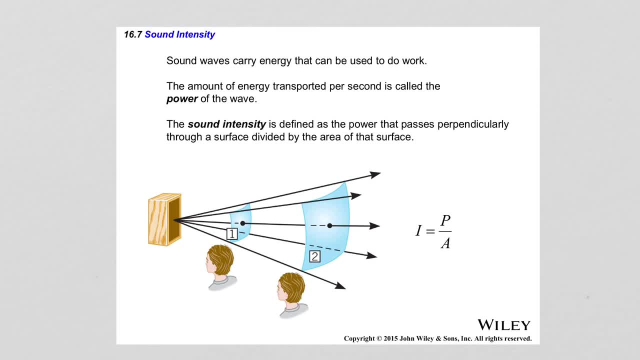 and the second one was the transportation of energy from one region in space to another region in space. So sound waves transport energy between two points in space. And to start this discussion, let's begin with the concept of sound intensity. First, let's define the power of a sound wave. 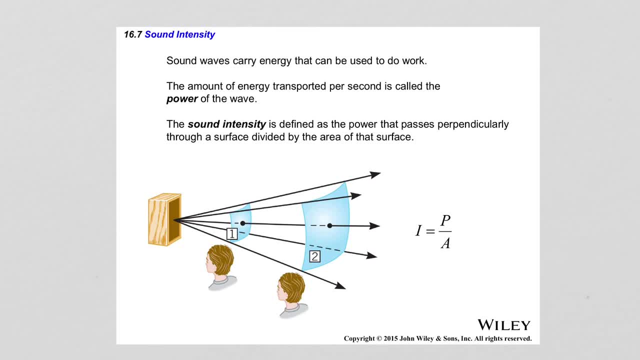 The power of a sound wave is the amount of energy that is transported per second and, of course, power, as in other areas of the course, is measured in watts. So then, if I take the power that is transported by the wave and I divide that by the surface area, 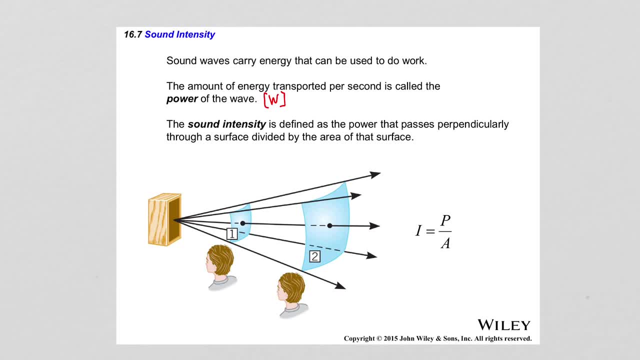 of a surface in space through which that wave passes. that's going to give me the sound intensity of that wave. So the sound intensity is defined as the power that passes perpendicularly through a surface divided by the area of that surface. So here is a sketch of such situation. 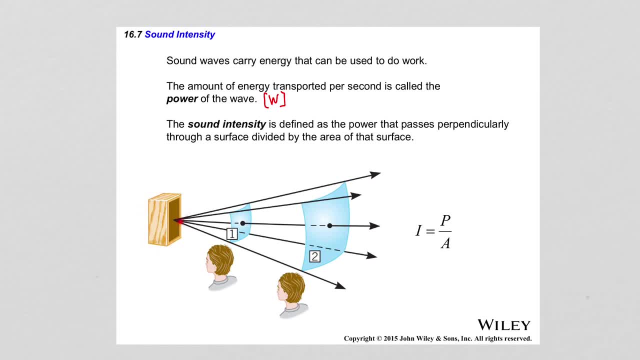 The sound source is a loudspeaker, The sound wave is generated, and so the sound wave passes through the surface here. So dividing the power of the wave by the surface area of this surface gives us the intensity at this point. Then the sound wave passes through this other surface here at point 2.. 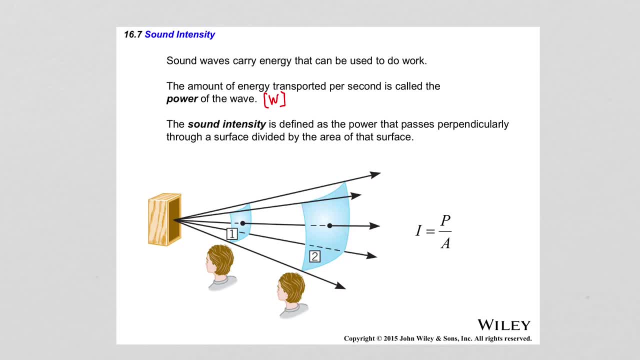 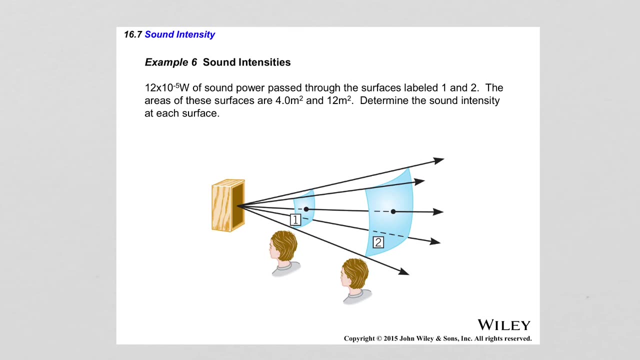 Dividing the power by the surface area of that surface gives us the sound intensity. at that point, The unit for sound intensity will be watts per square meter in the metric system. Let's look at the following example for calculating the sound intensity: 12 times 10 to the negative 5th power watts of sound are passed through a surface. 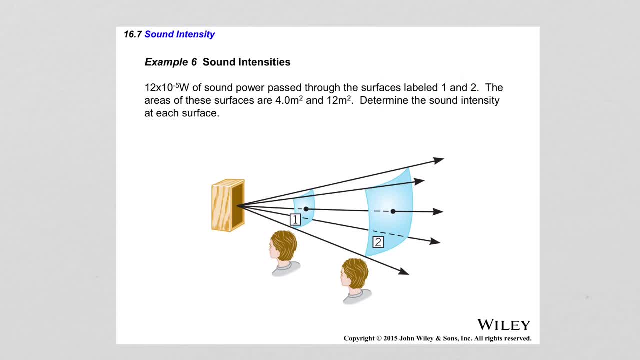 two surfaces labeled with 1 and 2.. The areas of those surfaces are 4 square meters and 12 square meters Determine the sound intensity at each surface. So, using the formula that defines the sound intensity, which was power divided by the surface area, 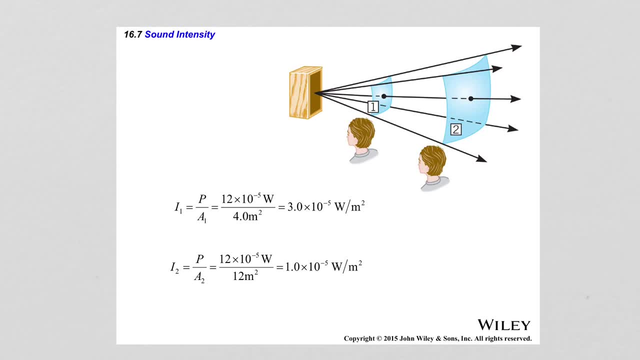 for the first point in space, the sound intensity is equal to the power divided by the surface area at that point. So that's 12 times 10 to the negative 5th watts. divided by 4 meters squared, That is 3 times 10 to the negative 5th watts per meter squared. 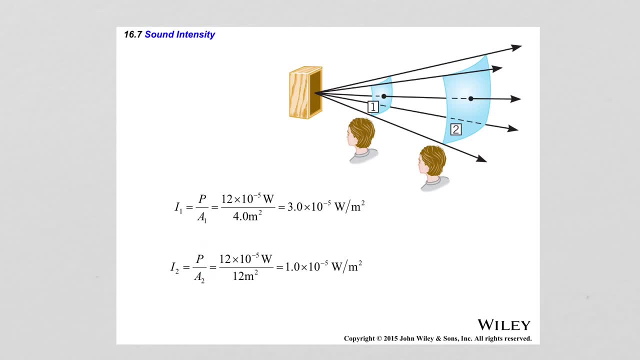 For the second surface we have power divided by the area of that second surface. So that is 12 times 10 to the negative 5th watts divided by 12 meters squared, Or that is 1 times 10 to the negative 5th watts per meter squared. 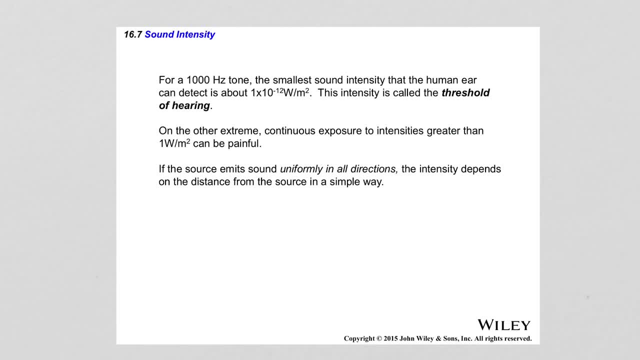 The human ear is capable of detecting sounds in the range from 20 Hertz to 20,000 Hertz, Depending on the intensity of the sound. there is a lower threshold beyond which the human ear cannot detect the sound. So for a 1000 Hertz tone, 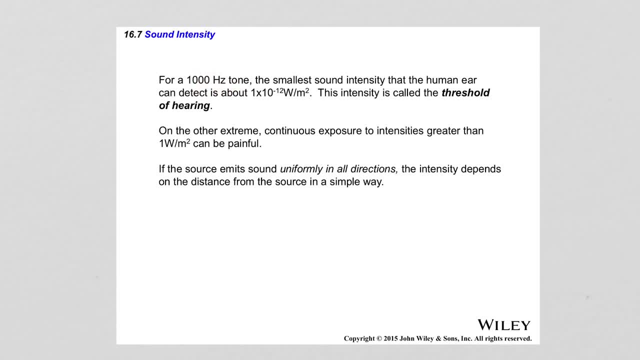 the smallest sound intensity that the human ear can detect is about 1 times 10 to the negative 12 watts per square meter. This intensity is called the threshold of hearing. So below that threshold the human ear cannot detect sounds. Now I discussed situations where the sound was basically propagating in one direction. 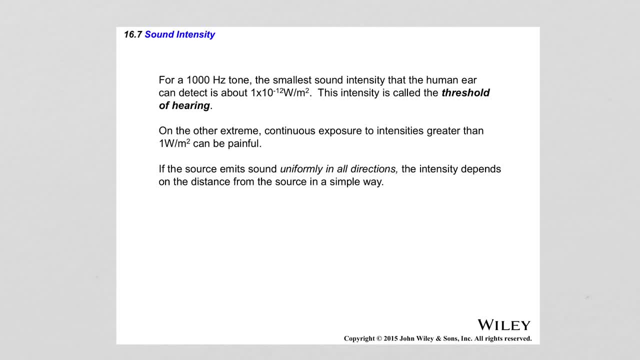 However, in reality, sound sources emit sound in all three dimensions of space, So sound sources are three-dimensional sources And, furthermore, if the sound source emits sound uniformly in all directions, the intensity depends on the distance from the source in a very simple way. 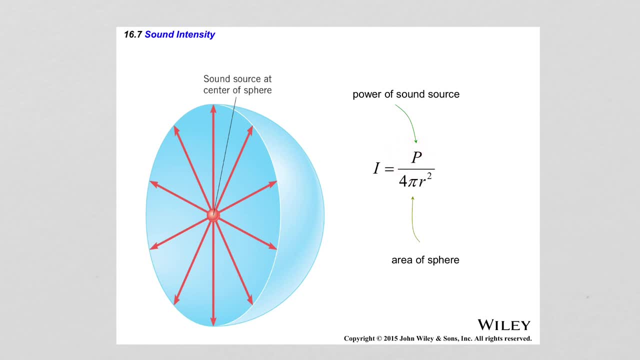 Intensity is equal to the power of the sound source divided by the surface area of a sphere. So why do we have a sphere here? Well, this is the sound source, and it emits sound waves in all directions, And so these sound waves, propagating in three dimensions, will. 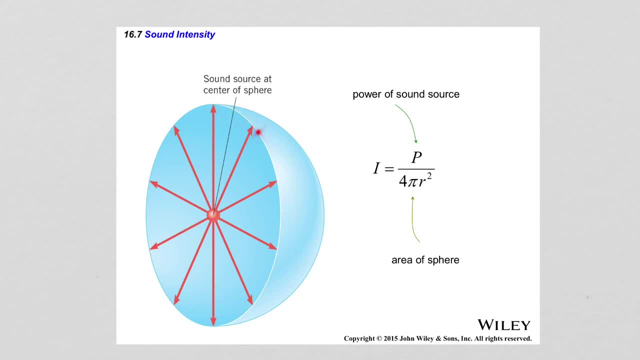 always pass through surfaces that are spherical, And so that's why we divide the power of the sound source by the surface area of the sphere to get the sound intensity at different points in space. Consider two sources that emit sounds with different sound intensities. 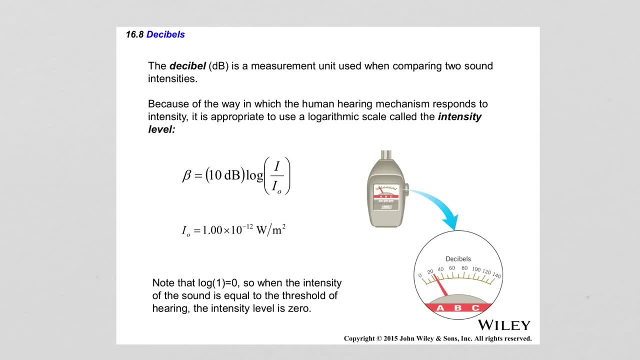 And we want to compare those two sound intensities. There is a way to do that, And to be able to do so we need to introduce a new concept, And that is the concept of decibel. Decibel is a measurement unit used when comparing two sound intensities. 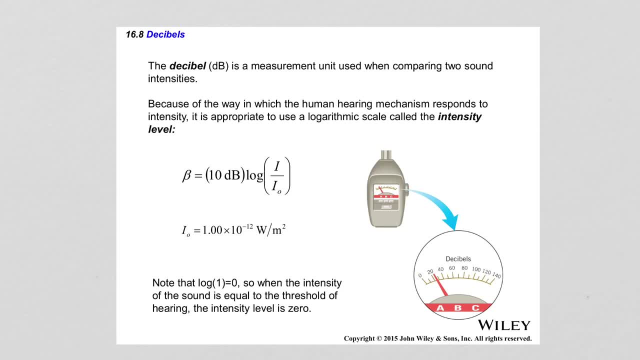 So, because of the way in which the human hearing mechanism responds to intensity, it is appropriate to use a logarithmic scale called the intensity level. The intensity level beta is equal to 10 decibels times the log of the intensity, the sound intensity emitted by the source divided by the threshold of hearing value. 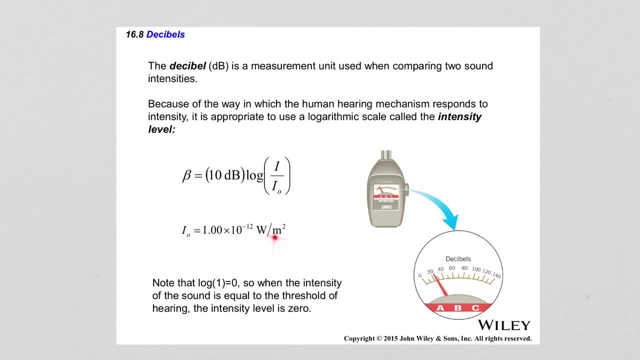 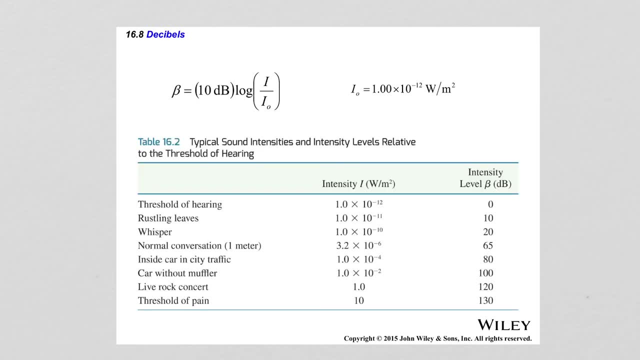 which is 1 times 10 to the negative 12 watts per meter squared. Here are some values for the intensity level of different sound sources. So the threshold of hearing has intensity of 1 times 10 to the negative 12 watts per meter squared. 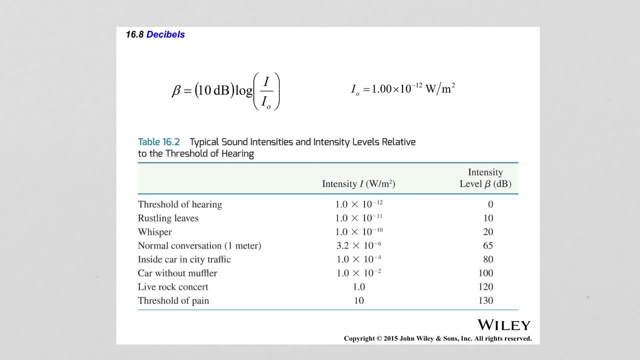 And then the intensity level is 0.. If we look at the intensity of sound for a normal conversation, that's 3.2 times 10 to the negative 6 watts per square meter. That corresponds to intensity level of 65.. The threshold of pain has intensity of 10 watts per square meter. 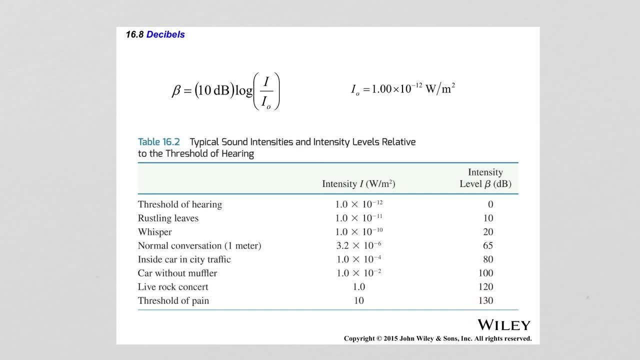 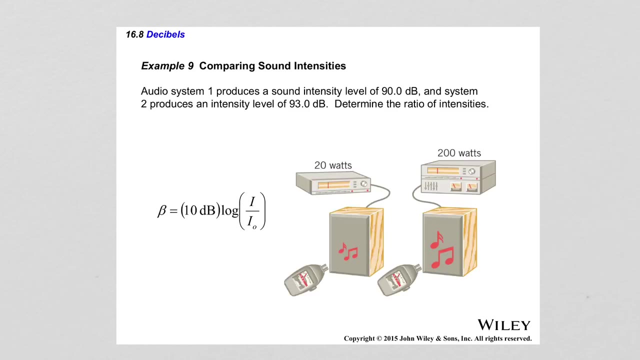 And the intensity level for that is 130 decibels. So beyond that, you would experience physical pain for sounds that have intensity level above 130 decibels. Now let's use the concept of intensity level to compare the intensities of two sound sources. 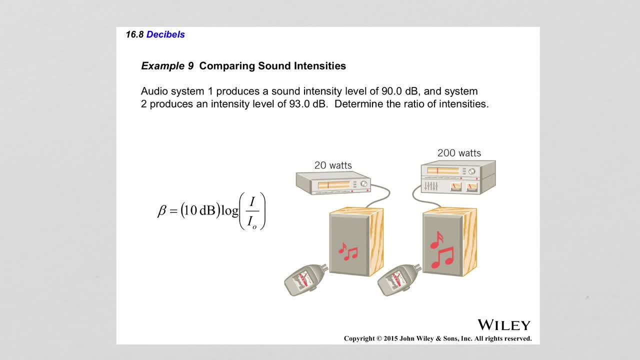 Audio. system 1 produces a sound intensity level of 90 decibels And system 2 produces an intensity level of 93 decibels. Determine the ratio of those intensities, So we are going to use the formula for the intensity level. 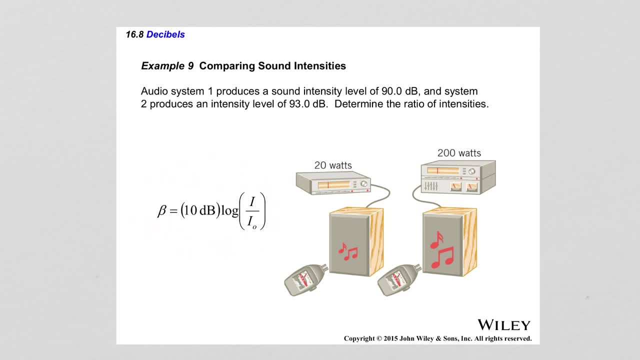 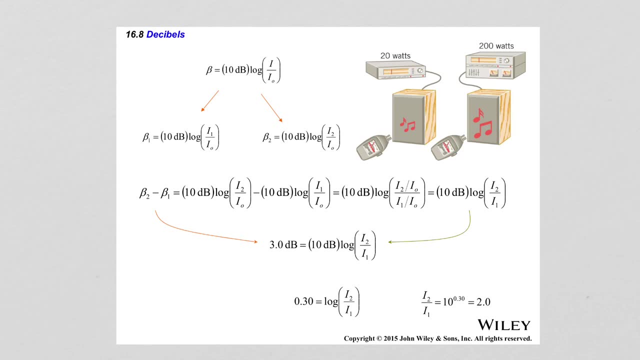 And we are going to write this formula In terms of each of the two audio systems. So that means we are going to index the parameters accordingly to indicate which audio system we are talking about. So for the first audio system, the intensity level beta 1 is equal to 10 decibels times log of I1 over I0. 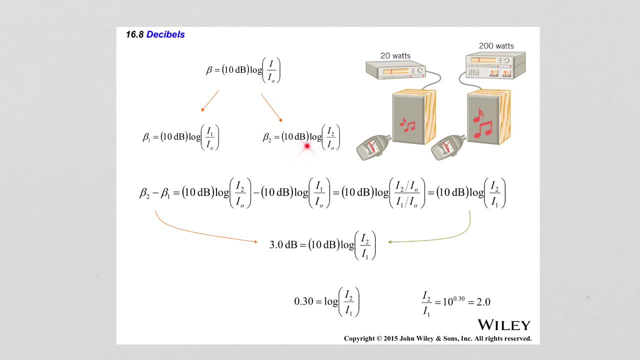 And for the second system, beta 2 is equal to 10 decibels log of I2 over I0.. Let's take the difference of those intensity levels. So the difference, beta 2 minus beta 1, is equal to 10 decibels log of I2 divided by I0. 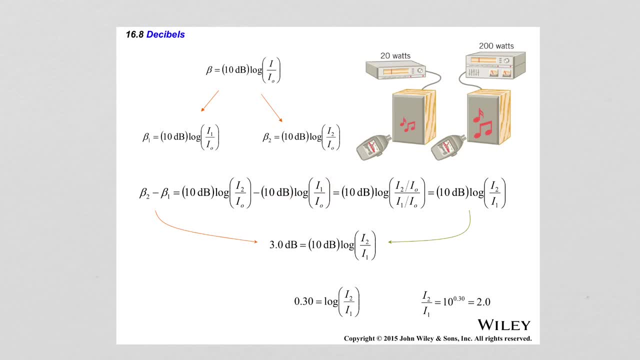 minus 10 decibels log of I1 divided by I0.. So the properties of logarithms tell us that this is equal to 10 decibels times log of I2 over I0, divided by I1 over I0. Or in other words, that is 10 decibels log of I2 divided by I1.. 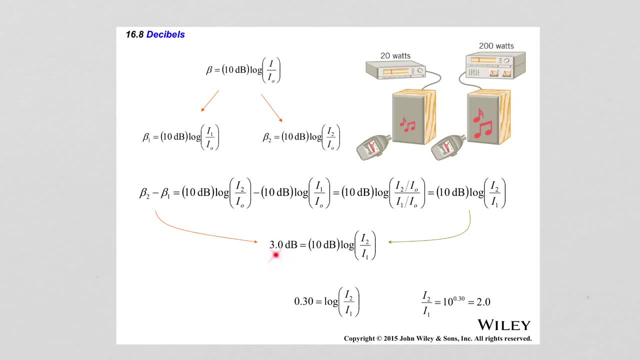 So the difference between the intensity levels is 3 decibels, And that is equal to 10 decibels times log of I2 divided by I1.. And so 0.3 is equal to log of I2 divided by I1.. 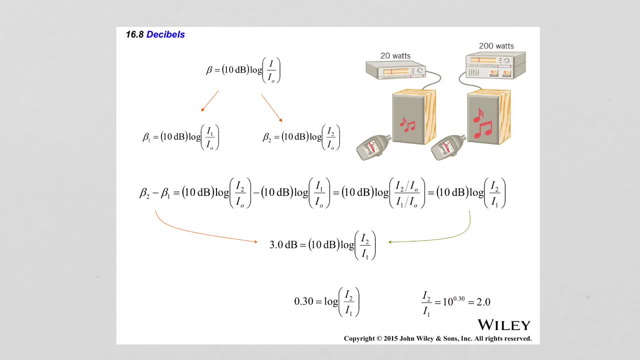 From where I2 divided by I1 is equal to 10, to the power of 0.3. Or that is 2.. So the ratio of the intensities for system 2 divided by system 1 is equal to 2.. Another interesting effect associated with sound is the Doppler effect. 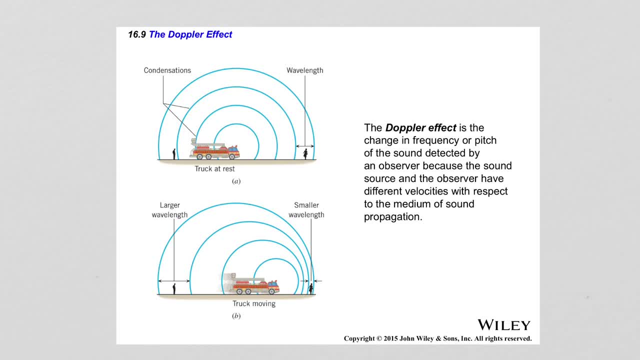 The Doppler effect is the change of frequency of the sound detected by an observer, because the sound source and the observer have different velocities with respect to the medium of sound propagation. Here is an interesting, simple illustration, rather, of the Doppler effect. In the first drawing here we have a sound source which is a fire truck. 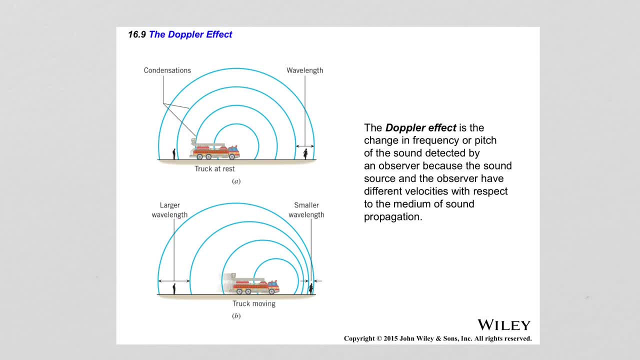 And two observers, one here and one here. The truck is at rest. the two observers also are at rest. The siren of the truck goes off. The siren of the truck goes off And sound waves are produced. So the sound waves propagate in all directions in space. 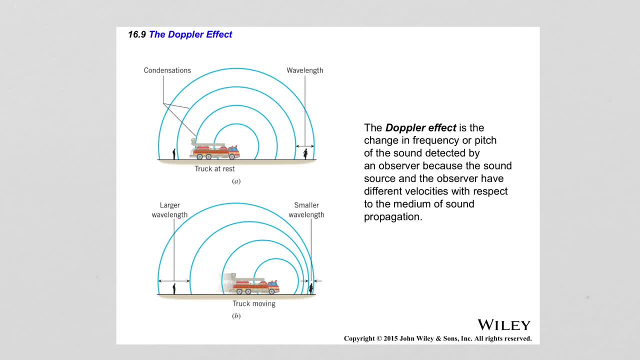 And we can map the crests of the sound waves. Or those are the areas where we have condensations of air molecules, And so these are the sound waves propagating away from the fire truck. The distance between two condensations is the wavelength of the wave. 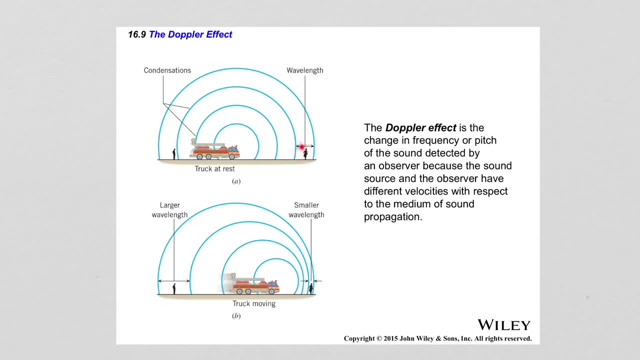 And so both observers, the one in front of the truck and the one behind, will hear the same pitch of the sound produced by the fire truck. Now let's have the fire truck move towards this observer here on the right. For the observer on the right. 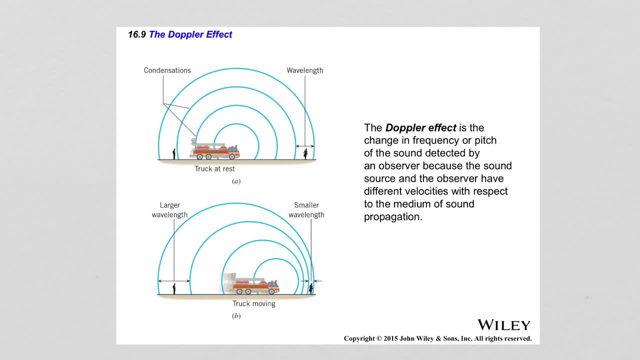 the wavelength of the sound will shorten And, as a result, that observer will perceive the frequency of the sound emitted by the fire truck as a higher frequency, So they will hear a higher pitched sound And you have probably experienced that in real life. 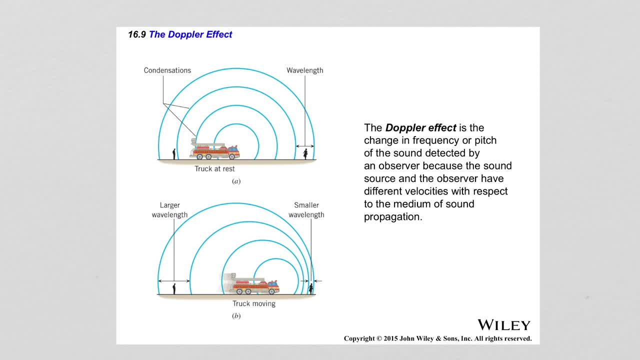 If you've ever been close to an ambulance that is approaching you, you know how it sounds, And then you also know that the sound of the ambulance is different once the ambulance passes you. So that's what happens for the observer that's behind the fire truck. 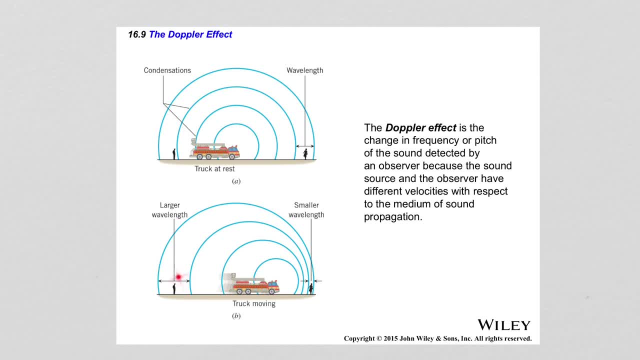 So as the fire truck moves away, the wavelength of the waves increases, Therefore the frequency for the observer decreases, And so he will hear a sound with lower pitch compared to the actual sound emitted by the fire truck. Let's explain those results. 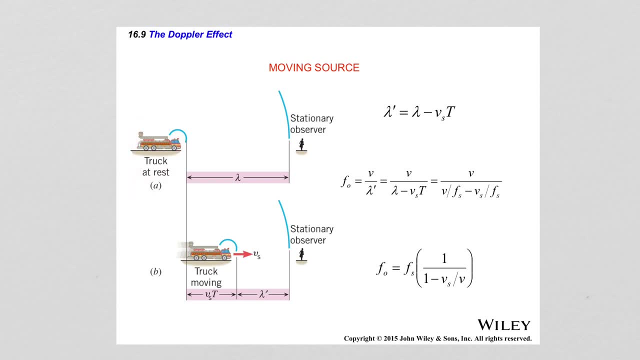 When the fire truck is at rest, the distance between two consecutive condensations is the wavelength of the wave lambda. But now, if the fire truck is moving with some velocity- Vs when the second condensation is created, the fire truck will already be a distance of V times T from the rest position. 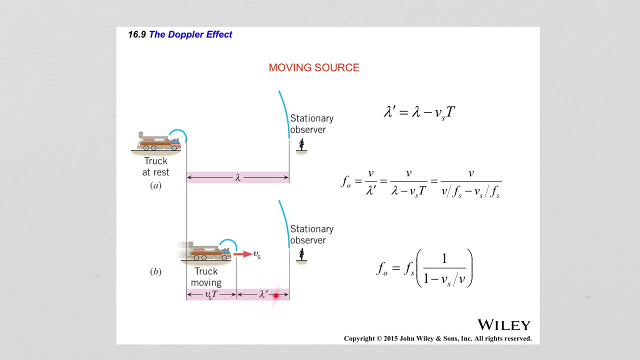 So therefore the wavelength of the wave produced will be equal to lambda prime, which is less than the wavelength when the fire truck was stationary. So then I can relate the wavelength lambda prime with the original wavelength lambda through the velocity of the fire truck and the time. 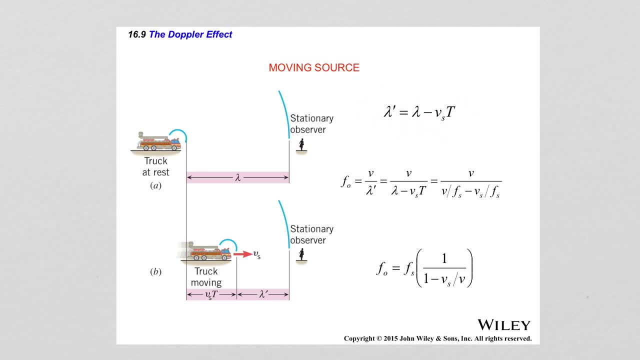 So that is the relationship here. On another hand, we know that the frequency that the observer will hear is equal to the speed of sound in air divided by the wavelength, And so after some algebra, we end up with this formula here that relates the frequency that the observer hears. 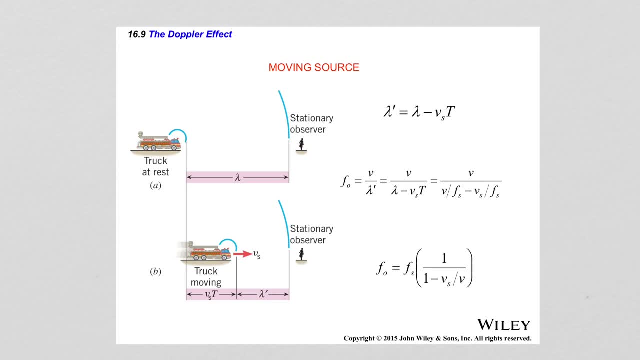 and the frequency that's emitted by the fire truck, The number that we get in the parentheses here is going to be bigger than one, which then results in the frequency heard by the observer being bigger than the frequency of the sound emitted by the fire truck. 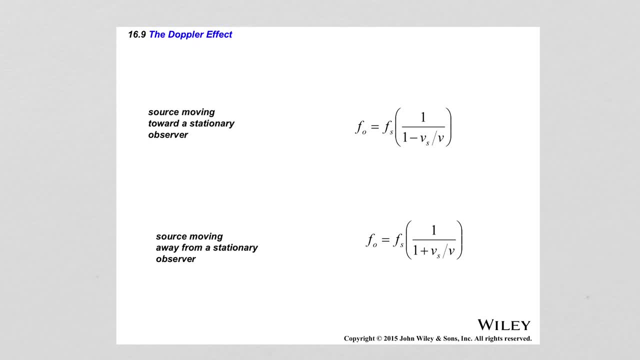 Similarly, we can calculate the frequency heard by the observer if the fire truck was moving away from them, And that is shown with this second formula here. In this case, the number in the parentheses is smaller than one, which then means that the frequency that the observer will hear 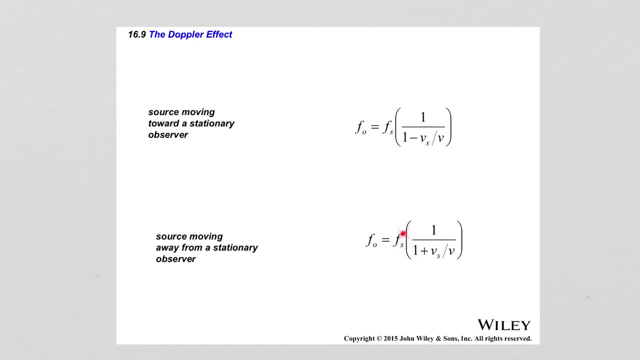 when the source is moving away from them will be less than the frequency emitted by the source. Here's an example problem of application of the formulas for Doppler effect when the source is moving and the observer is stationary. A high-speed train is traveling at a speed of 44.7 m per second. 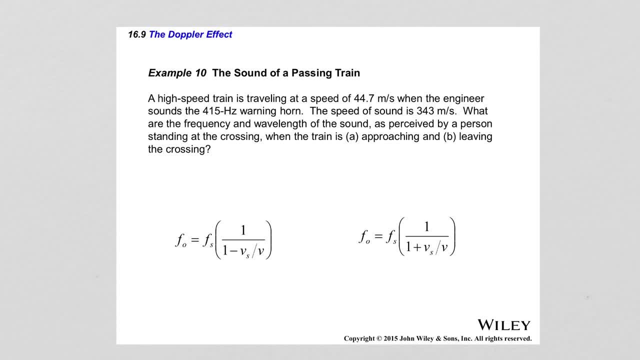 when the engine years sounds the 415 Hz warning horn. The speed of sound is 343 m per second. What are the frequency and wavelength of the sound as perceived by a person standing at the crossing when the train is approaching and when the train is leaving the crossing? 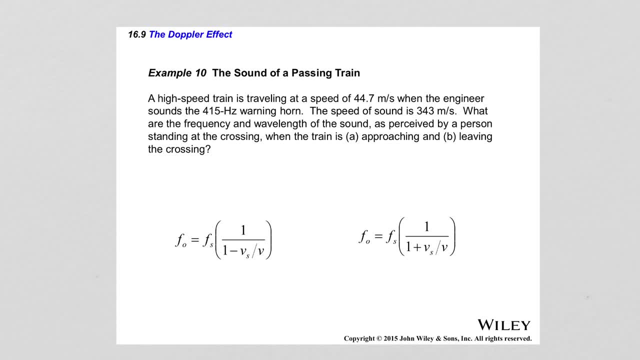 So here we have to use the two formulas that I discussed in the previous slide. The first formula was for the source approaching the observer, And the second one was for the source moving away from the observer, And so when the train is approaching the observer, 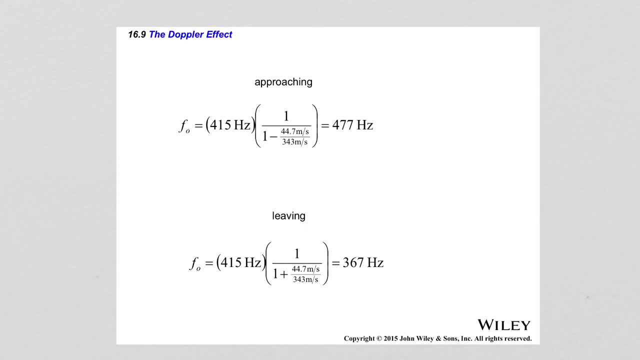 the frequency that the observer will detect is 415 Hz, that's the frequency of sound emitted by the train. times 1, divided by 1 minus 44.7 m per second, that is the speed of the train by 343 m per second. 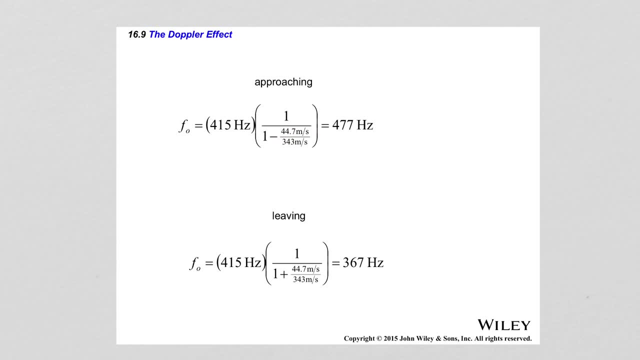 which is the speed of sound in air. As a result, the frequency that the observer detects is 477 Hz. Using the second formula, we can calculate the frequency that the observer detects after the train passes them, and that is 367 Hz. 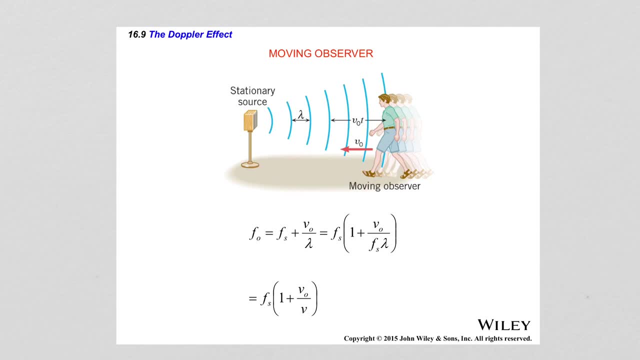 Now we have another situation in which the source is stationary but the observer moves towards the source. Now the frequency that the observer will detect will be different than the frequency emitted by the source. However, the formulas here are not the same as the formulas we discussed before. 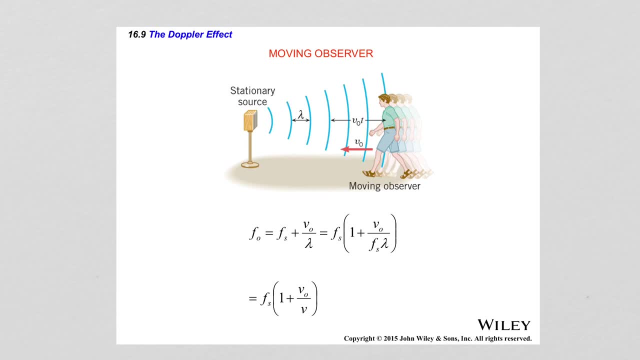 when the source was moving towards the observer. So here is our stationary source and it emits sound waves with wavelength lambda and frequency fs. Here is our observer who is walking towards the source. So, for a period of time t if the observer is moving with velocity vo. 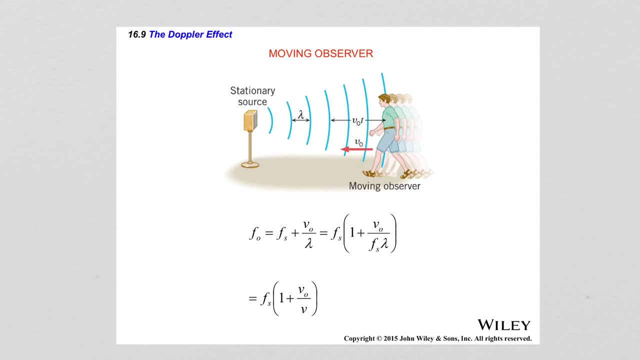 the distance that the observer will travel is v0 times t. So the observer will detect all the condensations that he would detect if he were stationary, plus an additional number which will be equal to v0 times t divided by lambda. And this here is just frequency. 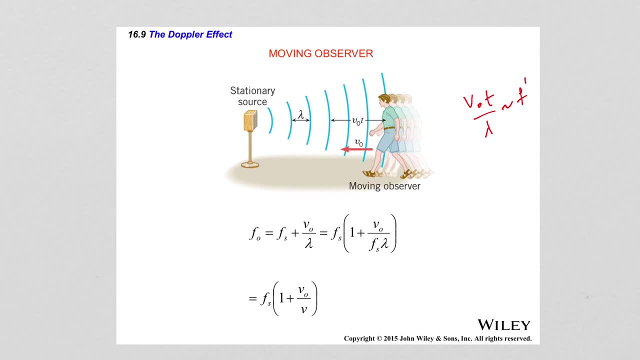 So for one second, then the observer will detect, simply v0 divided by lambda, extra condensations compared to if he were stationary. And so then, if I add the frequency of the source plus this extra number of frequencies due to the fact that the observer is, 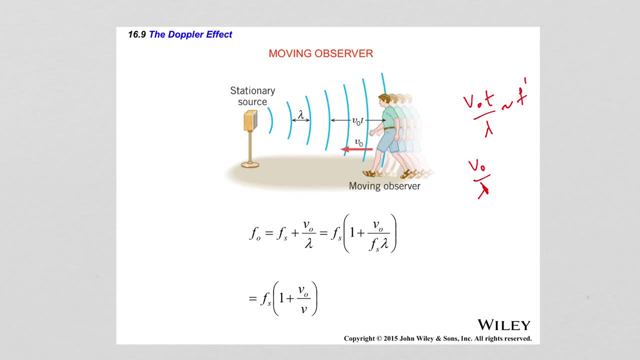 walking towards the source. after factoring out the frequency emitted by the source and applying the relationship between speed, wavelength and frequency, I will end up with this relationship, which relates the frequency that the observer detects and the frequency that the source emits. 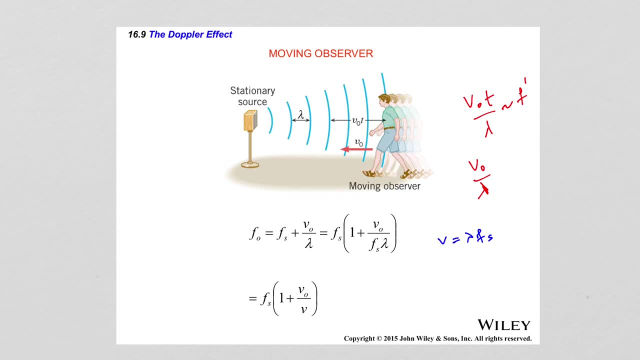 when the observer is moving towards the source, and the source is stationary. The number in the parentheses here is larger than one, and so the observer is going to detect frequency that is higher than the frequency emitted by the source, which is to be expected. 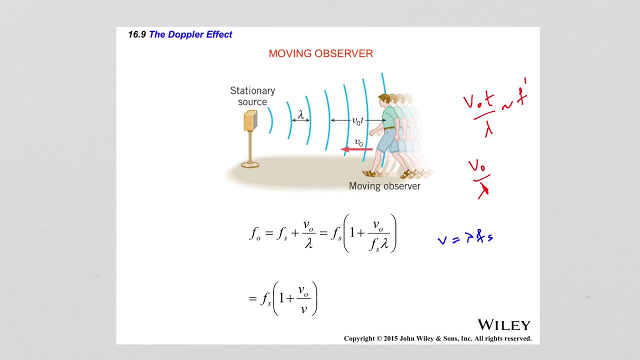 because, in a sense, this situation is similar to the observer being stationary and the source moving towards the observer, in which case we saw that the observer detects higher frequency. Of course, the same considerations can be used to calculate the frequency that the observer will detect. 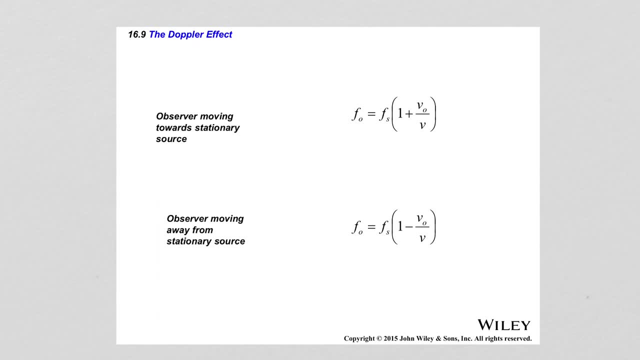 when they are moving away from the source, and this is given by the second formula In the parentheses. here we get a number that's less than one, which then means that the observer will detect frequency that is smaller than the frequency emitted by the source. 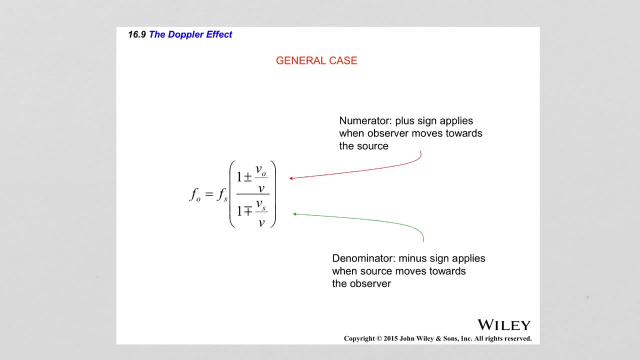 Finally, all of these can be combined into one general formula that looks like so: Here the pluses and minuses have to be selected accordingly to whether the source is moving or the observer is moving, in which directions they are moving, or if both are actually moving. 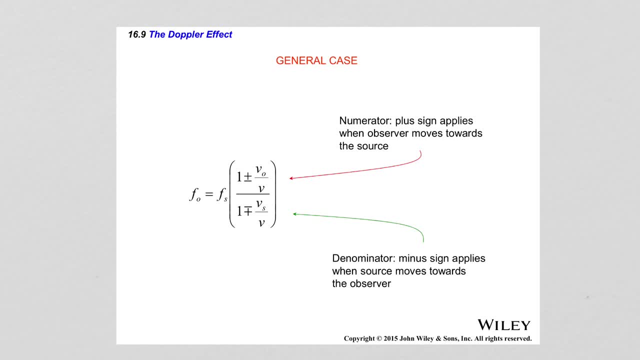 with respect to each other in which directions they are moving. So, for example, in the numerator the plus sign applies when the observer moves towards the source. That corresponds to this case. here. If we take the minus sign, that would correspond to the observer. 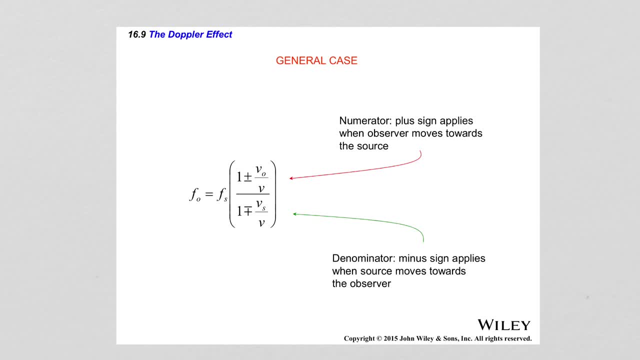 moving away from the source, And then in the denominator, the minus sign applies to when the source moves towards the observer, which corresponds to this case, and the plus sign corresponds to the source moving away from the observer, which corresponds to this case.